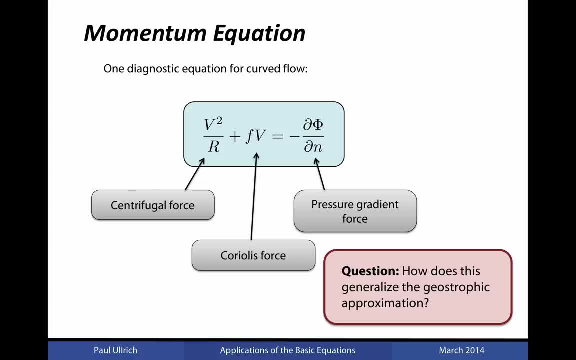 and pressure gradient force terms. Here the centrifugal force is described in terms of the square of the fluid's velocity divided by the radius of curvature of the flow. Recall: the radius of curvature is a quantity that describes the curvature an associated circle would have in case. it matches the radius of curvature of the flow. So we're going to use this equation to describe the radius of curvature of the flow. Recall: the radius of curvature is a quantity that describes the curvature. an associated circle would have in case it matches the curvature. an associated circle would have in case: 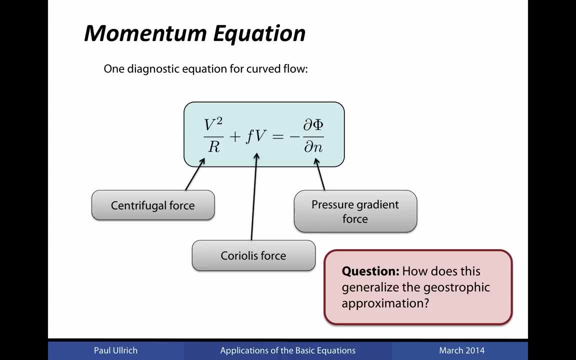 the curvature of the fluid parcel. The Coriolis force here is simply F times the flow velocity, and the pressure gradient force is simply the negative of the derivative of the geopotential height field in the normal direction. Recall that the normal direction is always directed here to the left of. 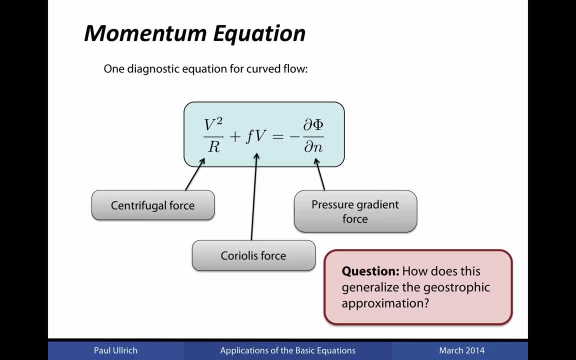 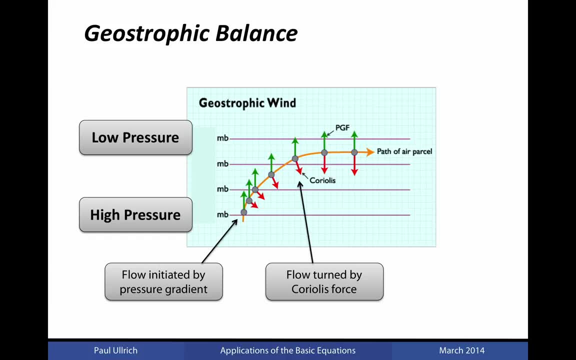 the flow velocity. So the first question that pops up is: how does this generalize the geostrophic approximation? Recall that the geostrophic approximation for the flow velocity is the pressure gradient force, For example. in this example we have a pressure gradient force. 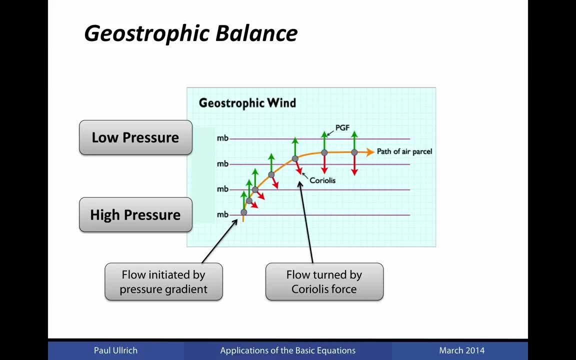 acting in opposite directions. The pressure gradient force in this case is acting northward and the Coriolis force is acting southward. The purple lines here denote lines of constant pressure gradient force, with pressure gradient decreasing towards the north Because of the modification associated with the Coriolis force, which causes the fluid parcel to turn to the right. we must have 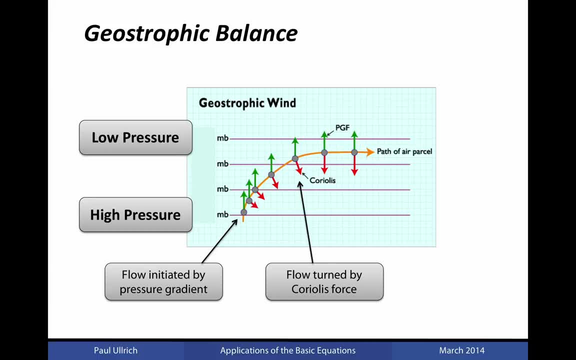 that the fluid parcel is moving to the right, The Coriolis force is acting northward and the Coriolis force acting eastwards in order for it to be satisfying geostrophic balance and, consequently, it is following along lines of constant geopotential. This balance, 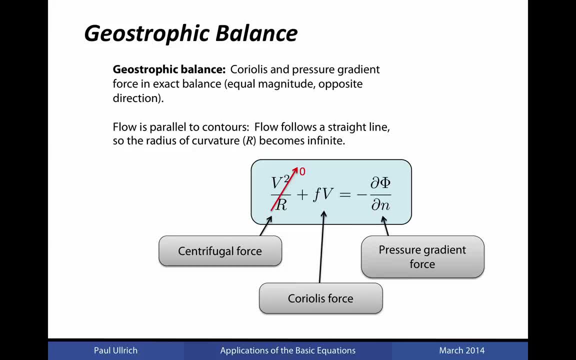 arises in the case of zero curvature, where the radius of curvature of the flow becomes infinite and corresponds to a straight line motion. Consequently, the centrifugal force term drops out from the three term balance relationship that we derived, and so we simply arise at a balance between Coriolis force and. 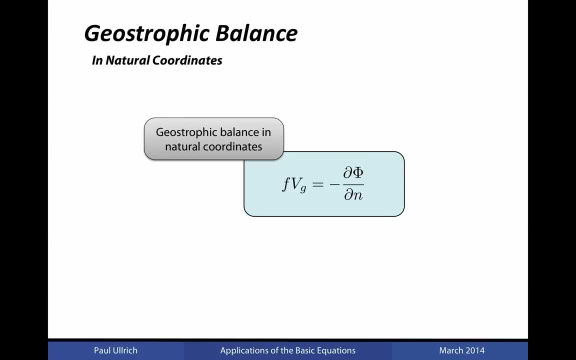 pressure gradient force In natural coordinates. then we can write this at balance as: F, V sub G, where the subscript G denotes geostrophic balance is equal to negative, di Phi, di n or the derivative of the geopotential height field in the normal direction. Diagrammatically we can depict the 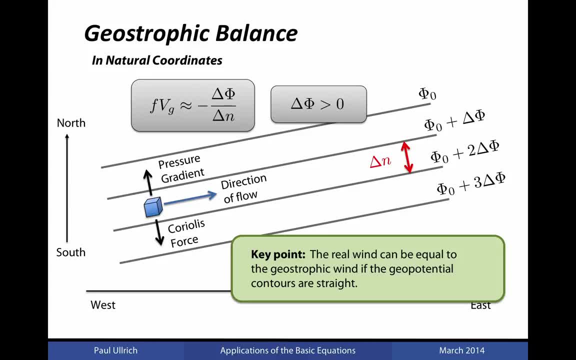 geostrophic balance for a case where the geopotential height contours are perfectly straight in the following way: The pressure gradient force in this case is directed up and to the left. The direction of flow for the fluid parcel is along lines of constant geopotential. 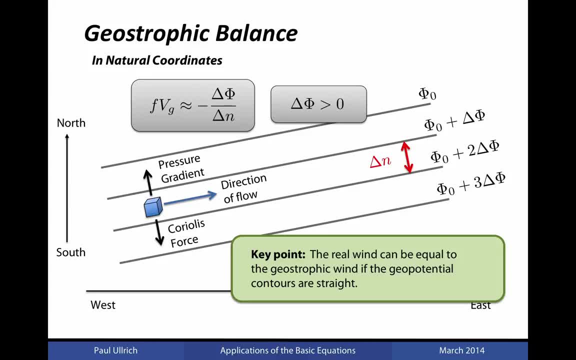 and the Coriolis force is directed to the southeast. The pressure gradient force in this case can be approximated through a finite difference. approximation, For instance, using a distance depicted here over the red arrows, Equal to delta n. This delta n denotes a coordinate distance in the normal. 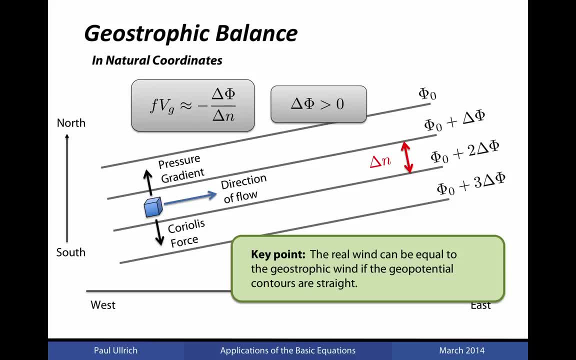 direction. Note that the normal direction in this case is to the left of the direction of flow. So for a coordinate distance, delta n, we have a change in geopotential delta Phi, and so the pressure gradient force experienced by the fluid parcel is then going to be equal to negative delta Phi over delta. 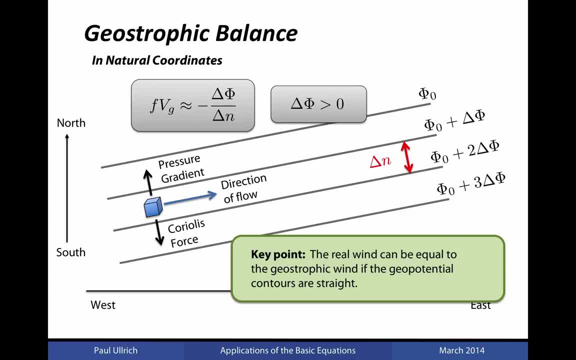 n. Using the relationship for geostrophic balance that we have had from the previous slide, we can then write this geostrophic balance as: F V sub G is approximately equal to negative delta Phi over delta n. In this case, the real wind or the real flow velocity of the fluid parcel is actually going to be. 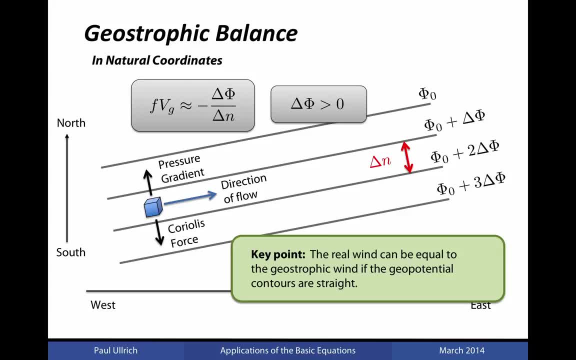 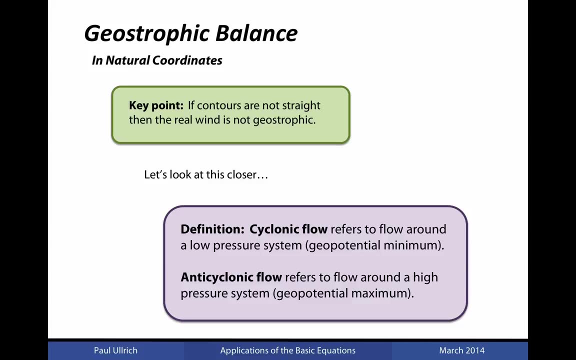 equal to the geostrophic wind speed if the geopotential contours are straight, Again corresponding to the case of an infinite radius of curvature and no centrifugal force experienced by the fluid parcel. However, if the contours are not straight, then the real wind is not geostrophic. So 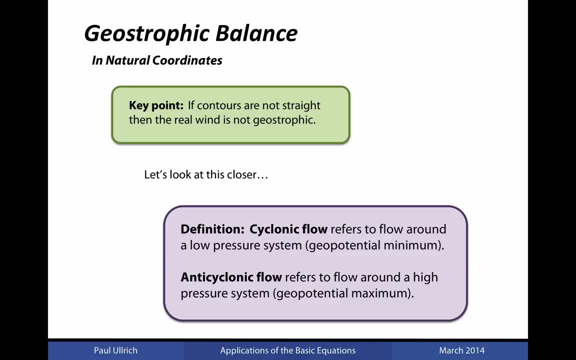 let's break this up into two possible flow regimes. We're going to define cyclonic flow as flow around a low-pressure system or flow around a geopotential minimum. This is associated, for instance, with flow around a tropical cyclone, extra-tropical cyclone or around an atmospheric trough. On the other, 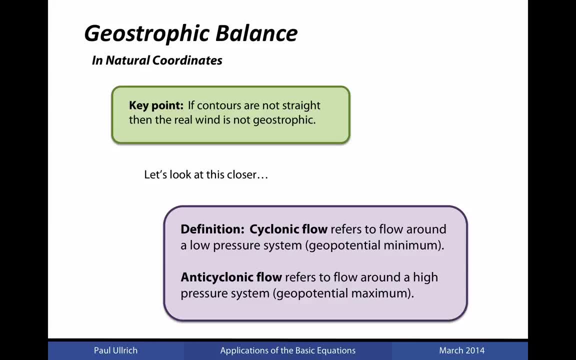 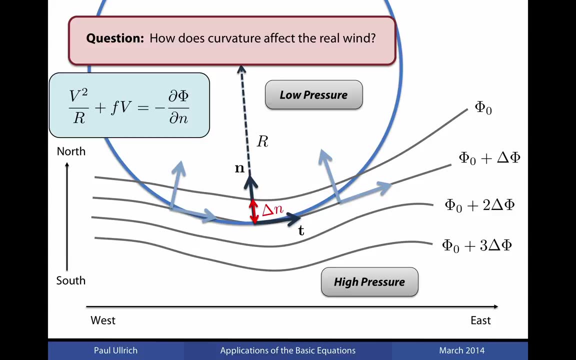 hand. anti-cyclonic flow refers to flow around a low-pressure system or a geopotential maximum. This is associated with flow around an atmospheric block or an atmospheric ridge, for instance. So in the case of flow around a low-pressure system, the circle that is associated 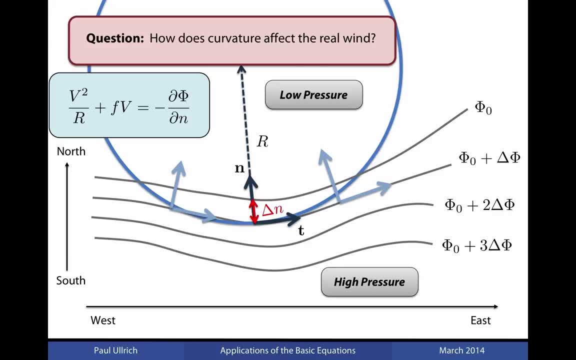 with the curvature of the flow then is centered around the low-pressure region. The radius of curvature is then associated with a normal distance that is positive. that is, the center of the circle is located in the same direction as the normal vector away from the fluid parcel. 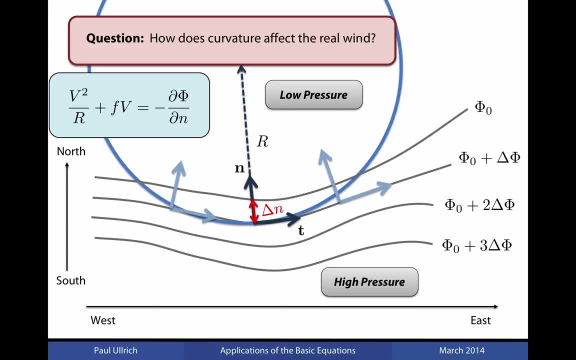 So curvature, in this case, then impacts the left-hand side of our expression. Now, instead of simply Coriolis force needing to balance the pressure gradient force, we have an additional term associated with centrifugal force acting on the fluid parcel. So in this case, when r is positive, we're going to have that the 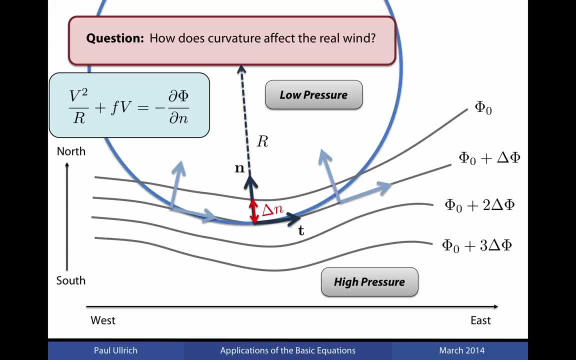 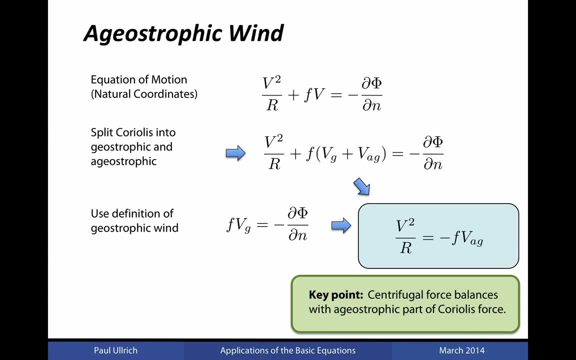 centrifugal force plus the Coriolis force together will balance the pressure gradient force experienced by the fluid parcel. Let's look at this in terms of the a-geostrophic wind. So the equation of motion that we had from the previous slide is our same three-term equation of 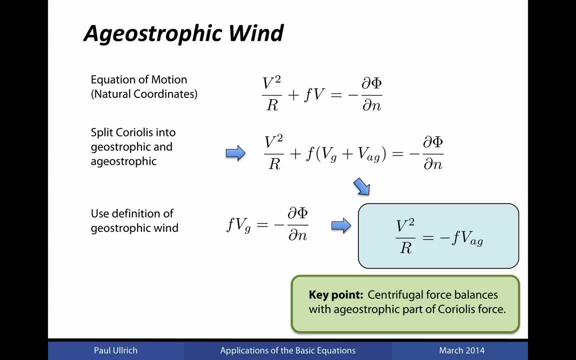 motion and natural coordinates. We can split this into a geostrophic and a-geostrophic flow, where the a-geostrophic flow is defined as the difference between the real wind velocity, capital V, and the geostrophic wind velocity Vg, that arises from the Coriolis. 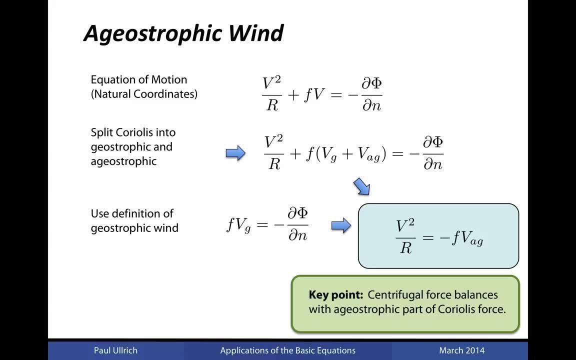 pressure, gradient, force balance. Substituting in V equals Vg plus Vag then gives rise to the second line in this derivation From the definition of the geostrophic wind here given. on the third line we can then write the a-geostrophic. 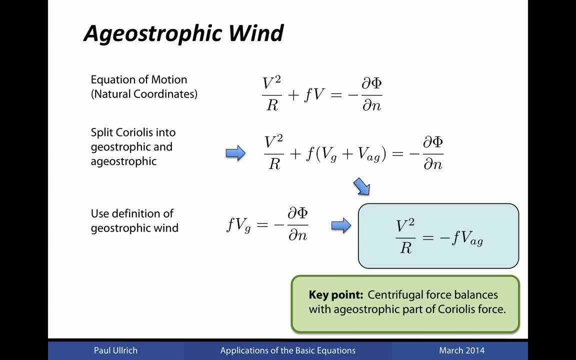 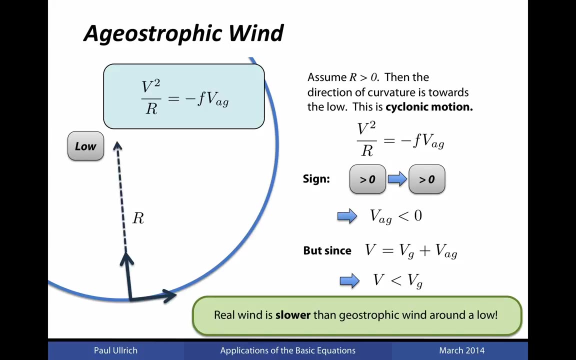 wind in terms of the centrifugal force that it then experiences. So, as we see from this expression shown here in blue, the centrifugal force is balanced by the a-geostrophic part of the Coriolis force. So let's consider the case of cyclonic motion. When, from the previous slide, we 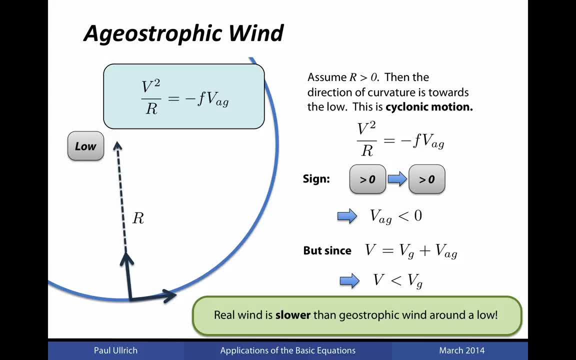 had. that centrifugal force is balanced by the a-geostrophic flow. that is the adjustment to the geostrophic wind needed in order to give the real wind velocity, Because flow is around the low we have, that the radius curvature is positive. 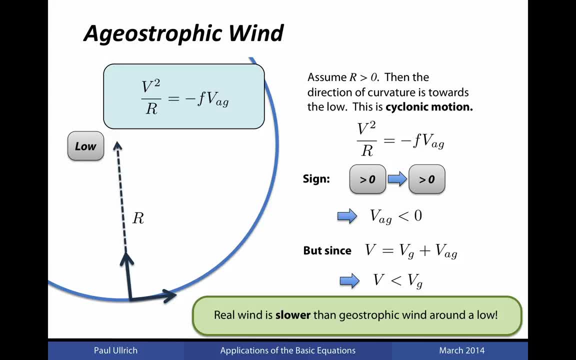 this means that the direction of curvature is directed towards the low, in the direction of the normal vector. Hence we have a sign on the left-hand side of this expression that is positive. that, then, must imply that on the right-hand side of this expression we also have a positive sign, Since F is 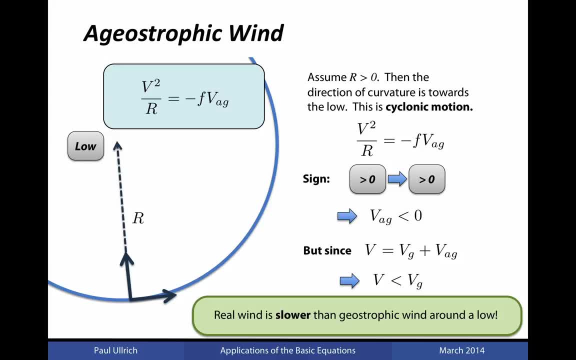 positive in the northern hemisphere and we have an additional negative sign on the right-hand side here. this implies that the a-geostrophic wind speed must be less than 0, or negative. However, since the total wind speed is equal to the geostrophic wind speed plus the a, 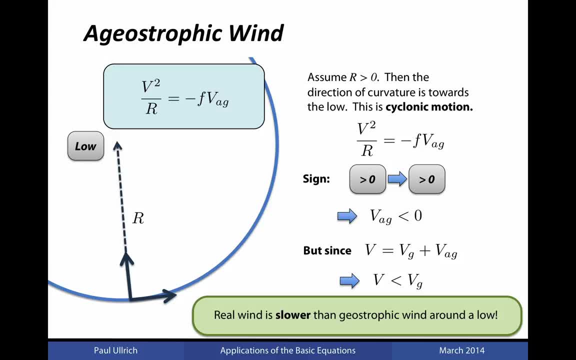 geostrophic wind speed. that must imply that the real wind must be smaller than the geostrophic wind speed. Consequently, the real wind is slower than the geostrophic wind when you are dealing with motion around a low-pressure region. This is analogous to what we pointed out in our last lecture about how the 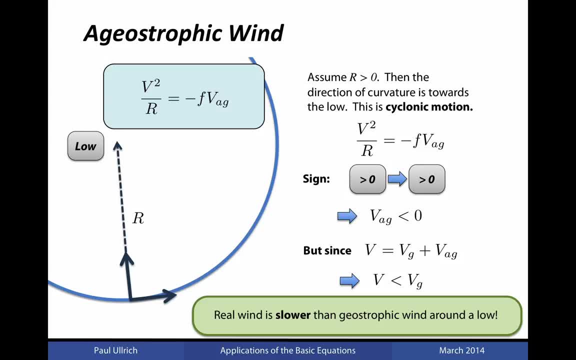 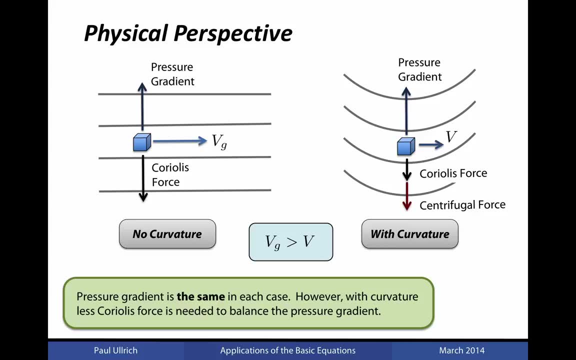 observed wind speeds did not agree with the geostrophic wind speeds when curvature was present. From a physical perspective, when we have no curvature, pressure gradient force is perfectly balanced with Coriolis force. These two vectors must have equal magnitude to one another and, in fact, the Coriolis force 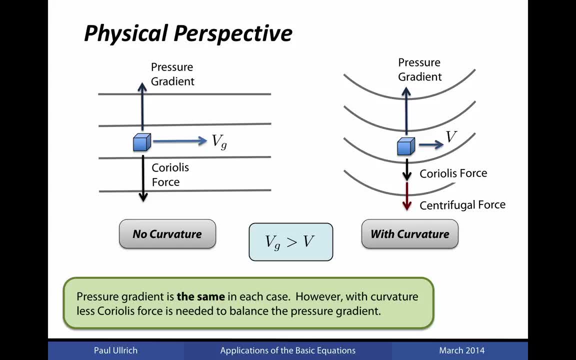 you'll recall, is exactly proportional to the flow speed of the fluid parcel. However, when curvature is present, we have that the sum of the Coriolis force plus the centrifugal force will balance with the pressure gradient force, and so you may be able to see that the sum of the Coriolis force plus the centrifugal force will balance with the pressure gradient force, and so you may. 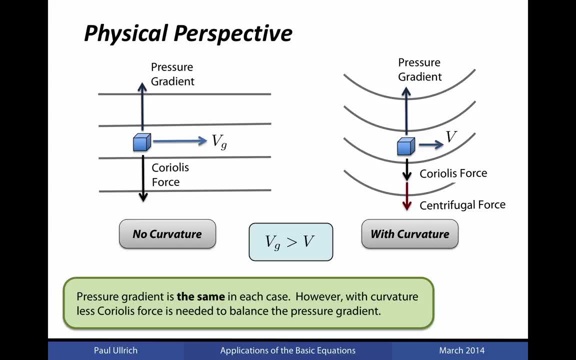 must have, that the real wind speed, which then determines the magnitude of the Coriolis force, must be weaker so that, when added to the centrifugal force, you have a balance with the pressure gradient force. In each case the pressure gradient is the same. Recall that we are imposing a pressure field that is 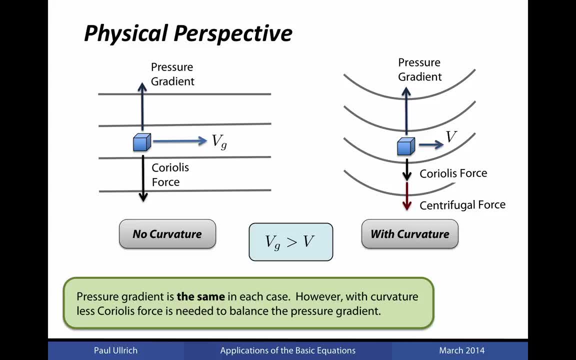 independent of the flow itself. so in each case, regardless of whether curvature is present or not, we have the same pressure gradient force. However, with curvature, we have the same pressure gradient force. However, with curvature, less Coriolis force is needed to balance the pressure gradient and 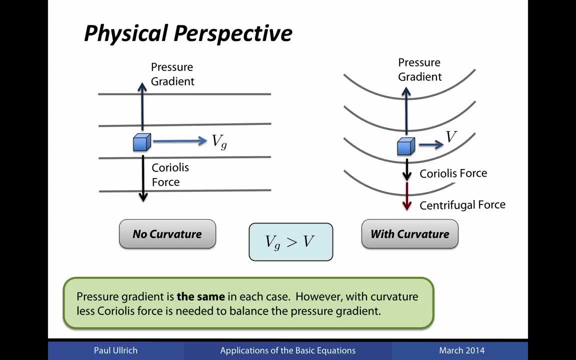 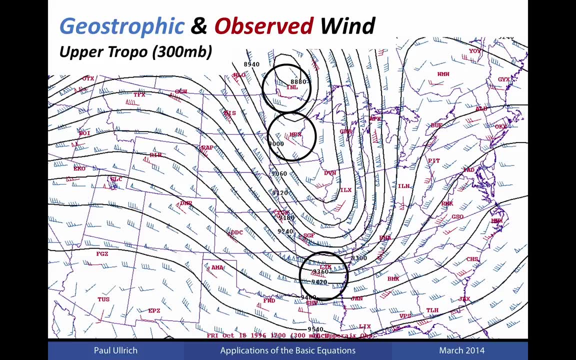 consequently, the flow velocity of the fluid parcel will be slower in the presence of curvature. This is observed in real life as well. Let's look at a few instances where we have flow around a low-pressure region, here highlighted with black circles. You'll notice that in each case, the red 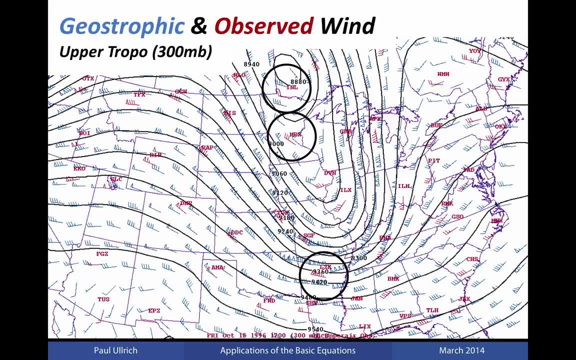 wind barb, which denotes the observed wind, is weaker than the associated geostrophic wind speeds denoted here in blue. In general, this is an. the geostrophic wind speed tends to overestimate the observed wind in each of these regions. If we look more close, for instance at LZh, at the 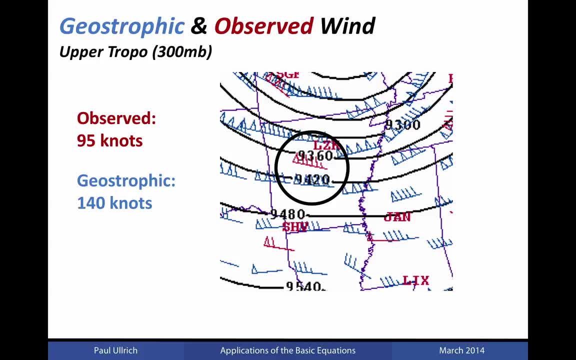 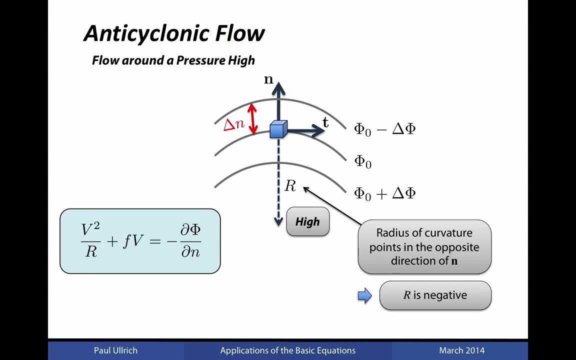 lower part of this diagram. the observed wind speed here is 95 knots and the geostrophic wind speed is a 140 knots. This adjustment is particularly severe in this case because the curvature in this region is very strong for the flow. Let's now consider flow around. 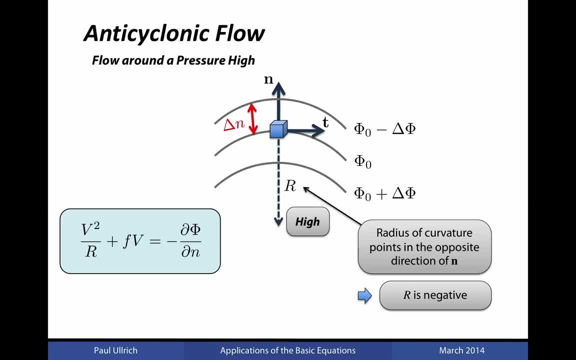 a high pressure region or the case of anticyclonic flow. In this case, the circle that approximates the motion of the fluid parcel appears below the fluid parcel or to the south of the fluid parcel and is centered around the high 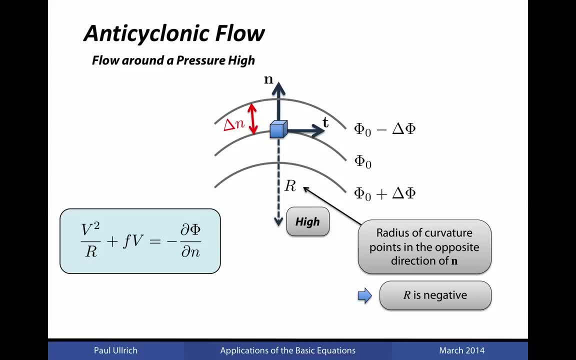 pressure region. Consequently, the radius of curvature, which is associated with the normal distance between the flow vector and the center of that circle, is going to be negative. That is, pointing towards, the center of the circle is in the opposite direction of the normal vector to the flow. So just 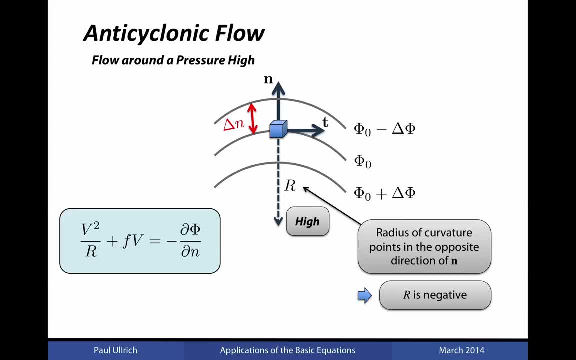 keep that in mind. then For cyclonic flow we have that the radius of curvature is positive and for anticyclonic flow the radius of curvature is negative. This is important in determining the impact of the centrifugal force on the fluid. 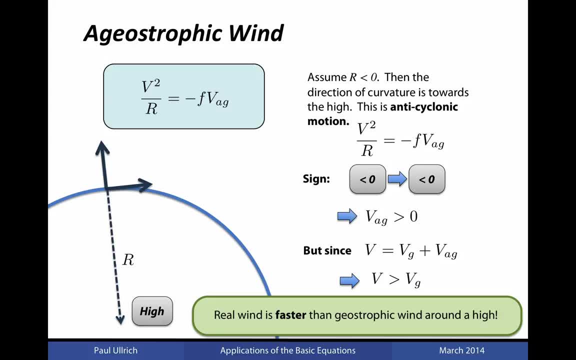 parcel Alright for anticyclonic flow with negative radius of curvature. the left-hand side of this expression will be negative. V squared will always be positive, so V squared over R must be negative in this case. This implies that the right-hand 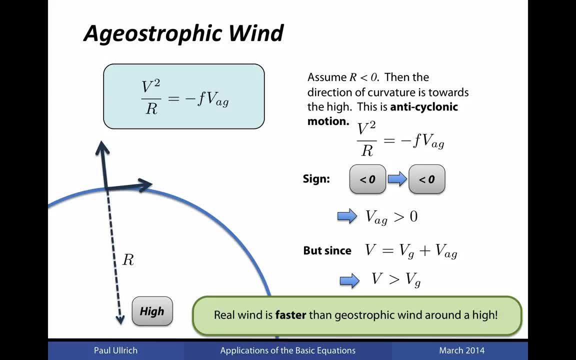 side is negative, and so in the northern hemisphere, where F is positive, we then must have that the a-geostrophic wind speed is positive, so that the signs of this expression are in agreement with one another. However, since the real wind is again equal to the geostrophic wind, plus the 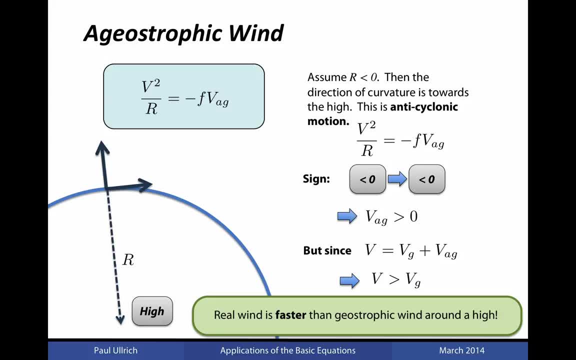 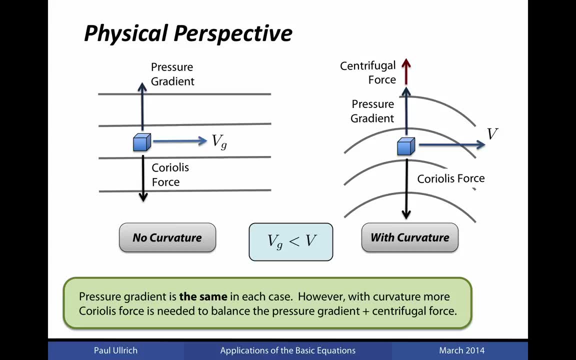 a-geostrophic wind, that implies that the real wind must be faster than the geostrophic wind. for flow around a high, Again from a physical perspective, we have, in the no-curvature case, pressure, gradient force exactly balances Coriolis force. However, in the case with flow around a high, the centrifugal force is: 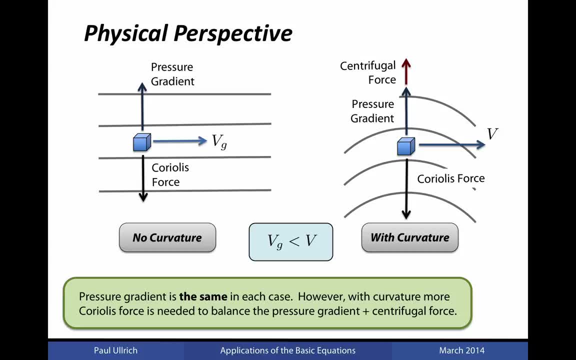 going to be directed in the same direction as the pressure gradient force, so these two vectors are additive to one another. The Coriolis force, which is then directed in the opposite direction to the pressure gradient force, must balance the sum of the pressure gradient and the centrifugal force and consequently must 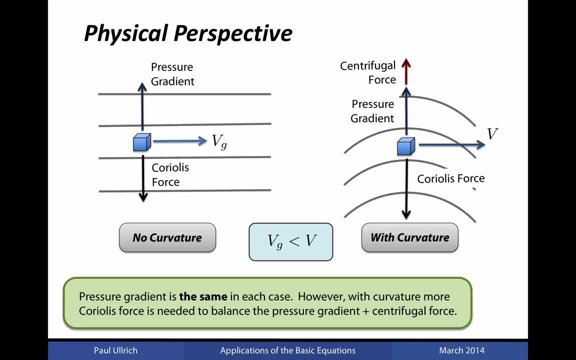 be longer than in the geostrophic flow case. So, even though pressure gradient is the same in each case, the curvature force, which is the pressure gradient force which is directed in the same direction as the pressure gradient force, requires a stronger Coriolis force and hence a faster fluid velocity, in order to 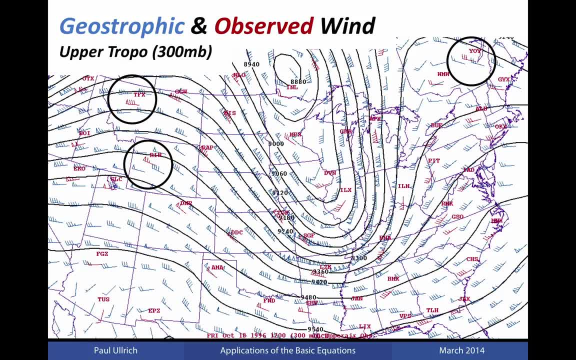 maintain balance. Let's look back at our diagram for regions where we have flow around a high, For instance, highlighted here in the three black circles, you notice in each of these regions that the observed wind is actually faster than the predicted geostrophic wind velocities. Let's, for instance, look at 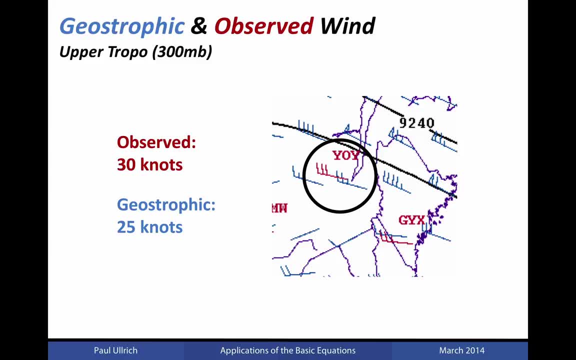 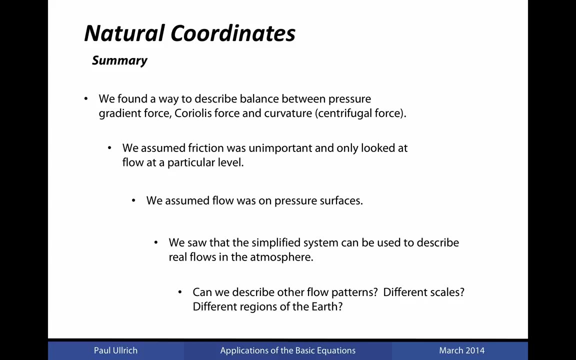 Y. In this case, the observed wind has a velocity of 30 knots and the geostrophic wind in the vicinity has a velocity of approximately 25 knots. So, again, this is consistent with our derivation on the previous slide. Alright, natural coordinates. in summary, We found a way to describe balance. 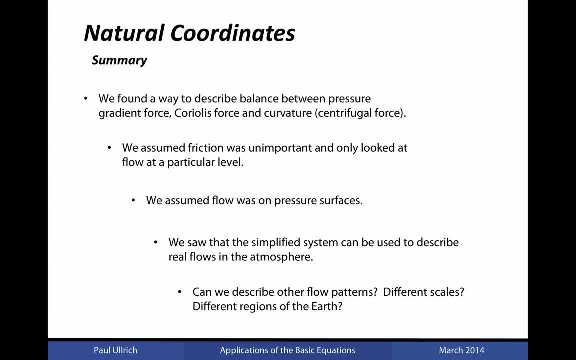 between pressure, gradient force, Coriolis force and curvature. so this generalizes the case of geostrophic flow by incorporating curvature and force in the flow. The curvature is then incorporated via a centrifugal force term. Note that this is a horizontal centrifugal force term analogous for 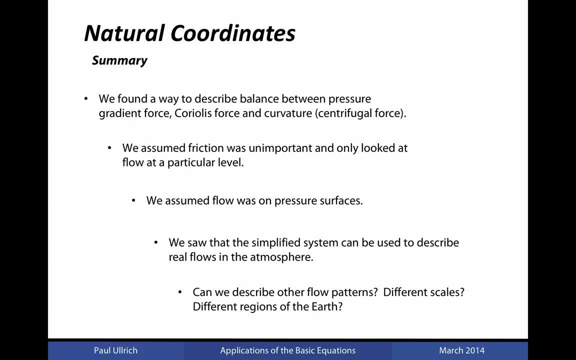 instance, to the force a object might experience if you were, for instance, twirling it in a circle on the end of a rope around your head. We assumed in this case that friction was unimportant and only looked at flow at a particular level. so we fix the pressure level at which we're performing our assessment. 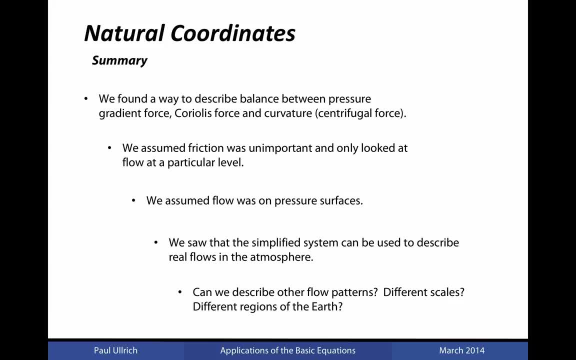 gradient force was then determined via a gradient of the geopotential field, We assumed the flow was constrained to these pressure surfaces and found that, using natural coordinates, we could derive a simplified system and a simplified equation of motion to describe real flows within the atmosphere and explain why there was a difference between the geostrophic prediction of flow velocity and 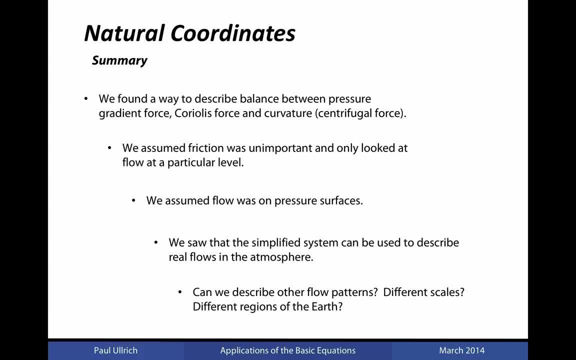 the observed prediction of flow velocity. So we can look at this a little bit farther in the case of balanced flow, and we can actually describe other flow patterns that occur at different scales and on different regions of the earth. Let's first start by looking at cyclostrophic 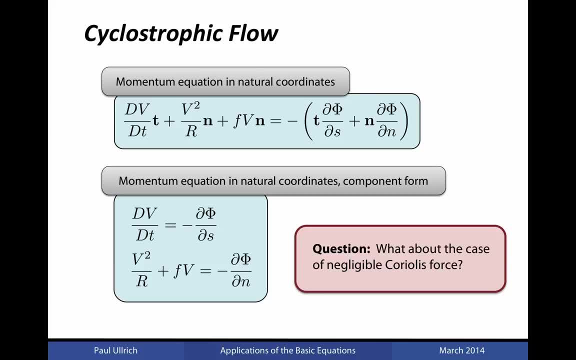 flow. This begins one of the three cases where we basically eliminate one of the terms from the three-term equation of motion that we just derived in natural coordinates, and we look at the force balance that results as a consequence of elimination of that term, The natural coordinate. 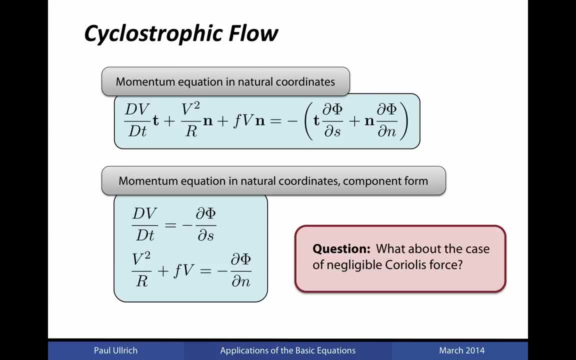 equation of motion is the force balance that results as a consequence of elimination of that term. The equation that we derived appears here at the very bottom of the slide, again incorporating centrifugal force, Coriolis force and pressure gradient force. Cyclostrophic flow is the special 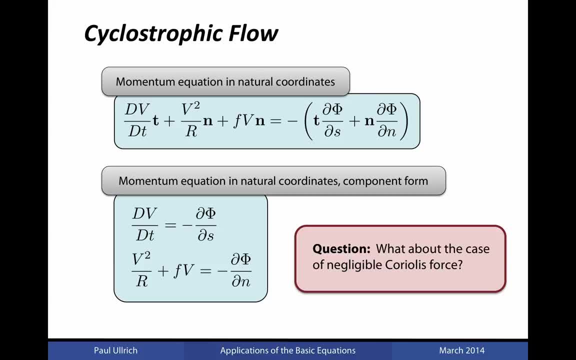 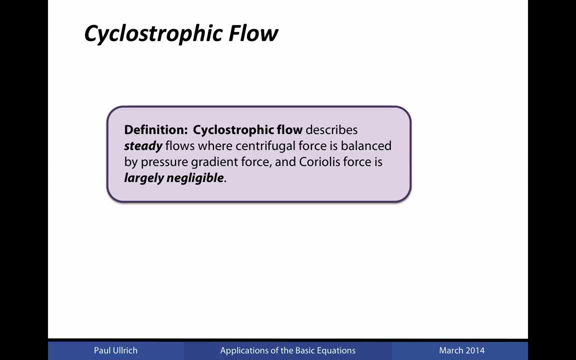 case where we have negligible Coriolis force. Negligible Coriolis force often occurs in cases where the horizontal scales associated with the problem are very small. So, for instance, one might anticipate cyclostrophic flow to pop up in the case of tornadoes. 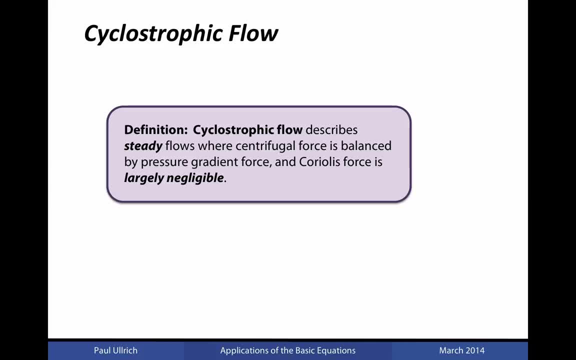 or dust devils, which have relatively small horizontal scales associated with them, but very large pressure gradients. Cyclostrophic flow describes steady flows where centrifugal force is balanced by pressure gradient force and Coriolis force is largely negligible. So in this case, 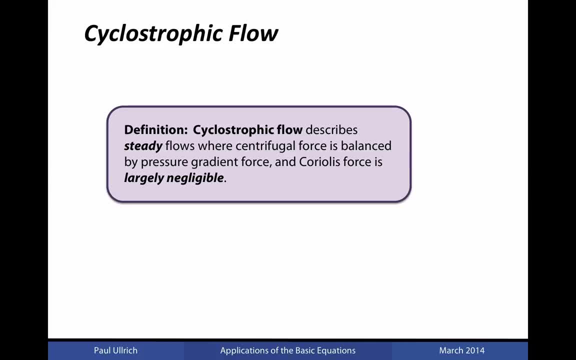 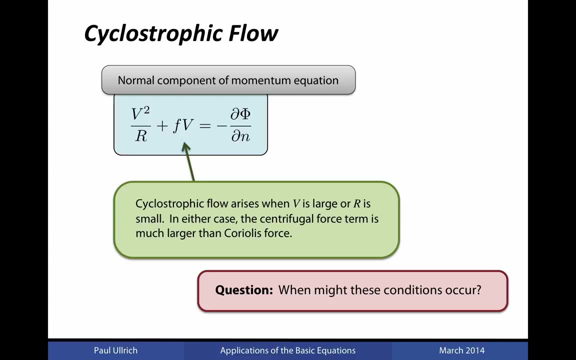 the primary mechanism by which pressure gradient force is balanced for a fluid parcel moving in a curved region is through the centrifugal force. So in this case this pops up again when v is large and consequently you have a large v squared compared to fv, or in the case where r is small. So, as mentioned, cyclostrophic flow tends to pop. 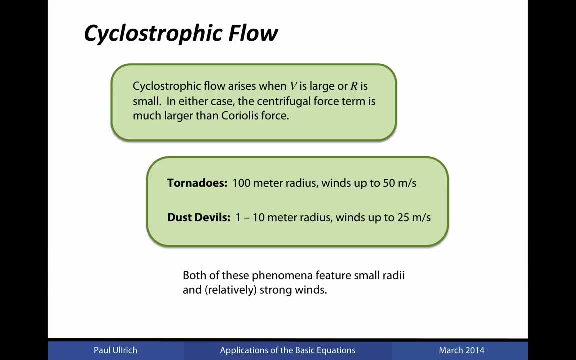 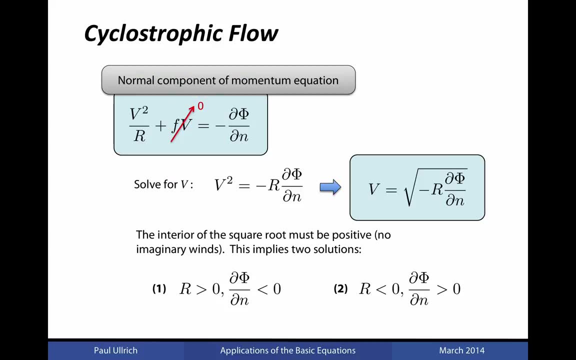 up for tornadoes and dust devils, with high wind speeds and small horizontal scales associated with the underlying phenomenon, So let's eliminate this term from the problem. We're going to look at the balance and then solve for the velocity experienced by the fluid parcel. Here we can. 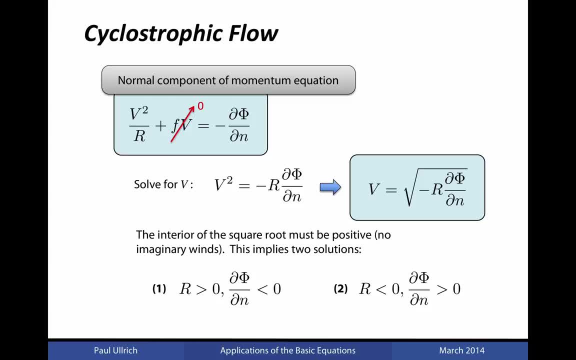 multiply through by the radius of curvature and take the square root of the expression. Hence the velocity experienced by the fluid flow is square root. negative r times the pressure gradient in the normal direction. The interior of the square root must be positive in order for 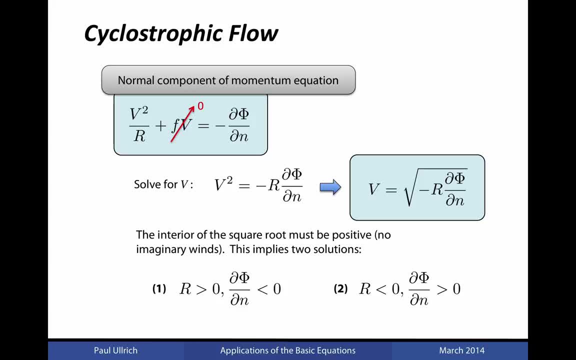 no imaginary solutions or no imaginary roots to arise from this equation. This implies that only two solutions are physically possible: Either the radius of curvature is positive and the pressure gradient force is negative, or the radius of curvature is negative and the pressure gradient- sorry- the derivative of the geopotential height in the normal direction. 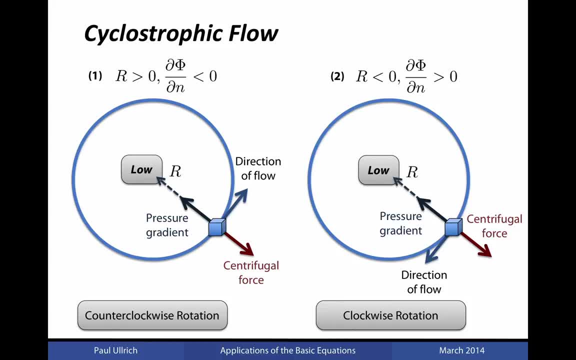 is positive. Diagrammatically, these two look as follows: Either you have a direction of flow which is in the counterclockwise, as one might anticipate for typical large-scale flows around low-pressure regions. Consequently, the radius of curvature direction is pointed in the same direction as the normal. 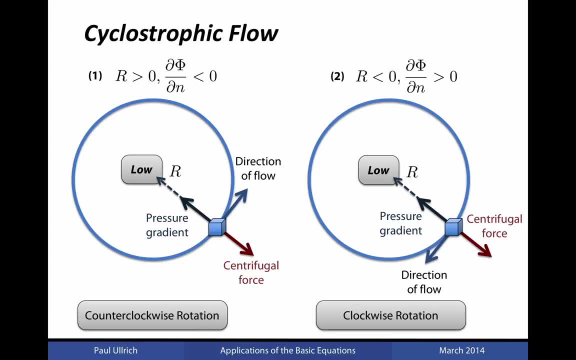 vector to the flow and it is balanced by the centrifugal force which is pointed outward from the circle. So centrifugal force always acts away from the circle. It's attempting to push the fluid parcel away from the center. The pressure gradient force also is always directed. 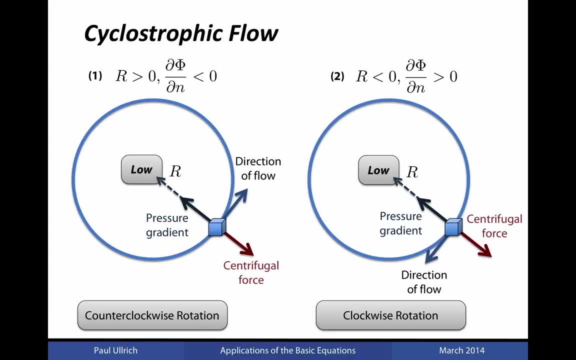 towards the interior of the lobe, and this gives rise to a direction of flow which is counterclockwise. In the second case, the force balance is actually identical, but what flips is the direction of flow, Because the normal direction is then to the left of the direction of flow or more. 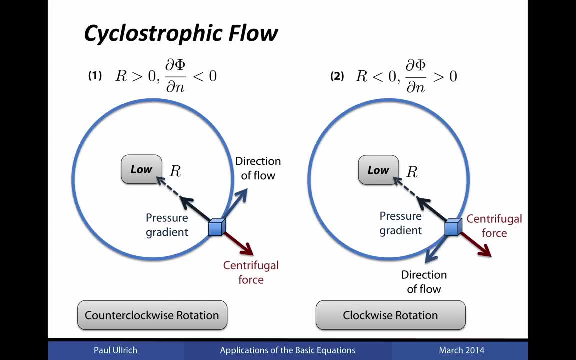 generally is to the left of the direction of flow. then the pressure gradient increases as you move in the normal direction, But the radius of curvature in this case must be directed towards the center of the circle in order for this to be a physically legitimate case. So we actually end up with the exact same physical configuration in each case. 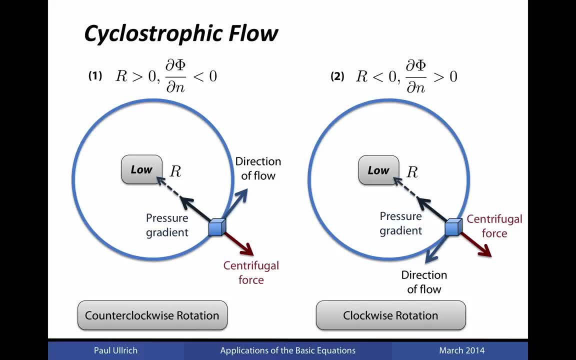 except on the left-hand side you have counterclockwise rotation of the fluid parcel, whereas on the right-hand side you have clockwise rotation of the fluid parcel around the lobe. So interestingly, there's no preferred direction of the fluid parcel for the cyclostrophic flow case. 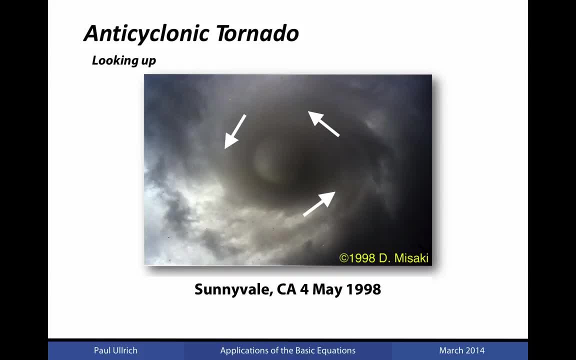 This is contrary to large-scale flows where, if you recall, for extratropical cyclones, for instance, or tropical cyclones, which are relatively large-scale phenomenon, you always have in the northern hemisphere counterclockwise motion around the low-pressure region. However, in 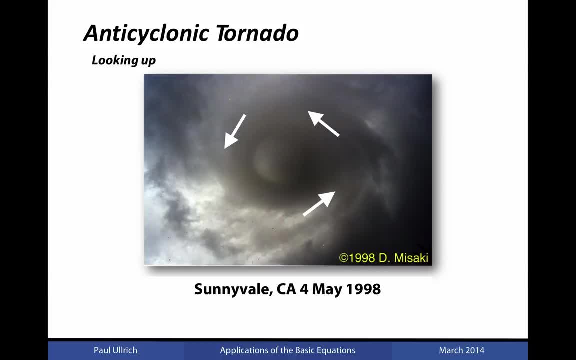 the case of tornadoes, which are dominated and described by cyclostrophic flow, you can actually have anti-cyclonic motion. The counterclockwise rotation associated with tropical cyclones and exotropical cyclones always appears when you're looking down on the object from space. 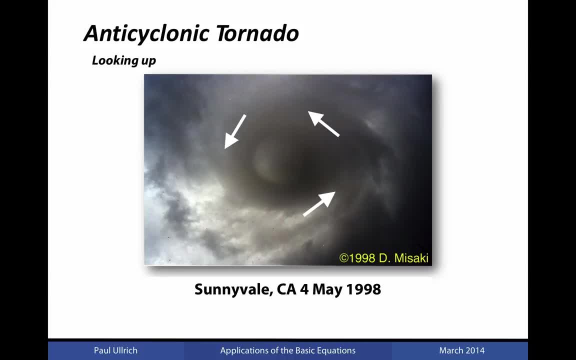 In this image shown here, which is a picture of a tornado taken from the ground looking up through the feature, we see counterclockwise rotation looking up, which corresponds then to clockwise rotation looking down on the object. Hence, this tornado is actually an anti-cyclonic tornado. 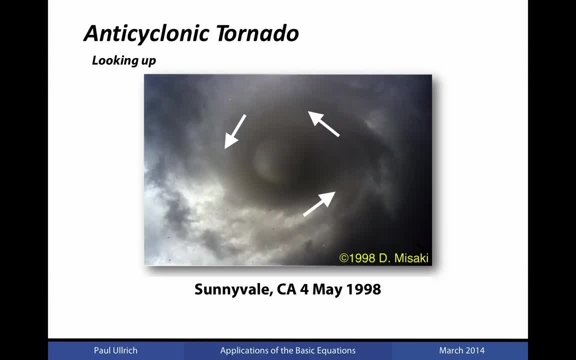 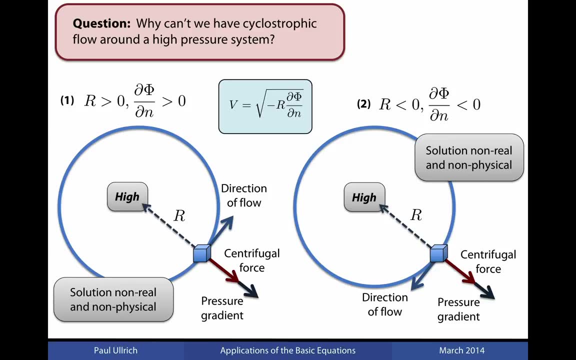 That is, the flow is clockwise about a low-pressure region. So why can't we have cyclostrophic flow around a high-pressure system? Let's consider the two possibilities for force balance that would be experienced by a fluid parcel if there was a high at the center of the direction of the stream flow of the flow. 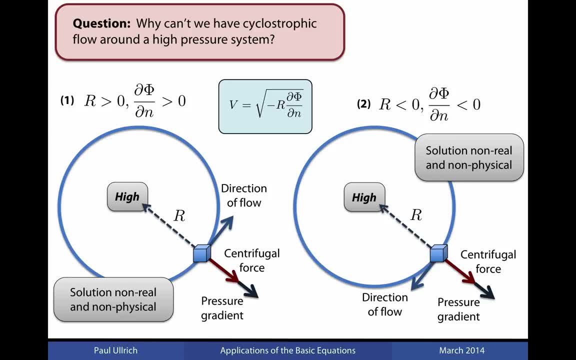 direction of the fluid parcel. So if our direction of flow, for instance, is counterclockwise around a high-pressure region, centrifugal force is always directed away from the circle, so it is directed outward, and the pressure gradient is also directed outward. 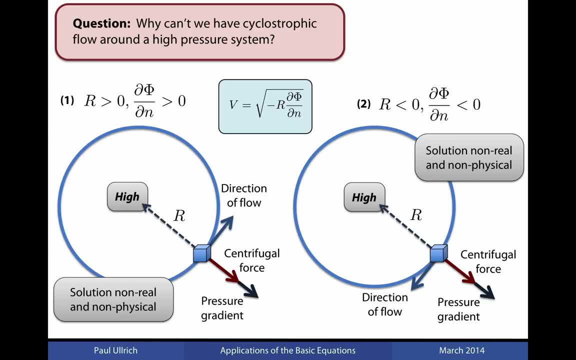 Because Coriolis force is negligible. we have no force in this force balance diagram which can counteract the sum of the centrifugal and pressure gradient forces being experienced by the fluid parcel. So this is an unphysical force balance On the right-hand side. here we consider an opposite flow direction. 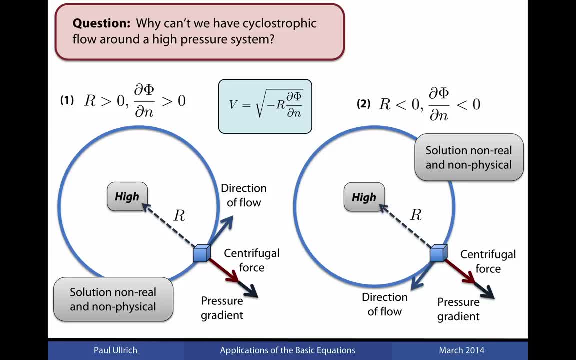 In this case, again, centrifugal force is directed outward, and pressure gradient force, which goes from high to low, is also directed away from the high. Again, we basically have the exact same configuration of force vectors experienced by the fluid parcel, and so the fluid parcel will be ejected from the high rather than being in balanced. 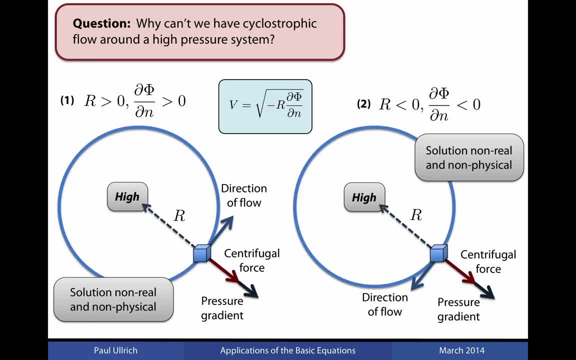 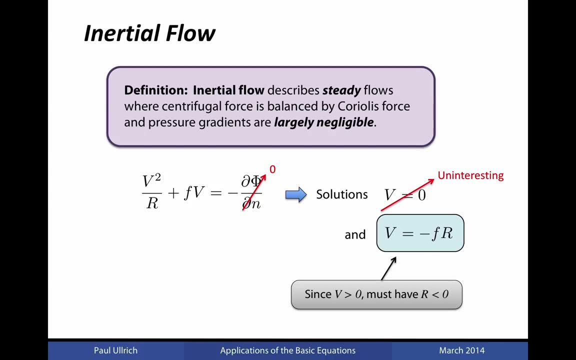 motion around the high. So in each case there is no physical solution. that arises from the case of force balance, and so cyclostrophic flow requires that the flow be around a low-pressure region. Alright, let's consider the third case of balanced flow. 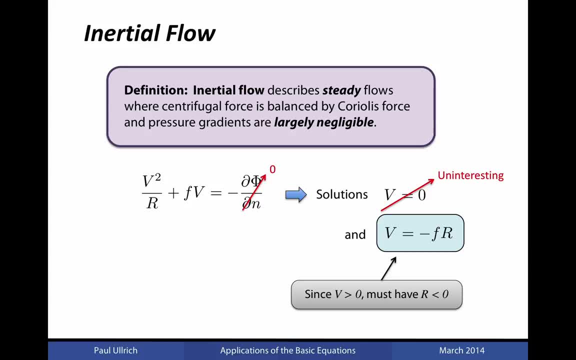 So recall, so far we've talked about geostrophic flow, which is balance between Coriolis force and pressure gradient force. The second case, which is cyclostrophic, 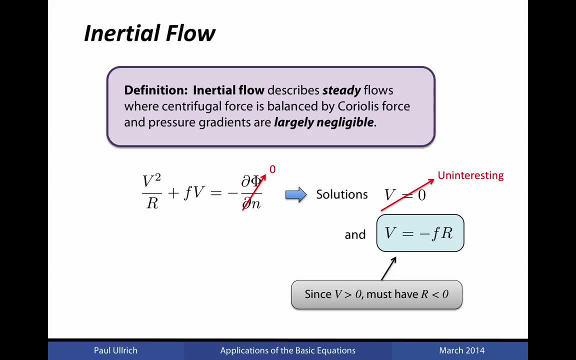 flow corresponding to the balance between centrifugal force and pressure gradient force. The last case involves a largely negligible pressure gradient. or, more formally, inertial flow, describes steady flows where centrifugal force is balanced by Coriolis force and pressure gradients are largely negligible. 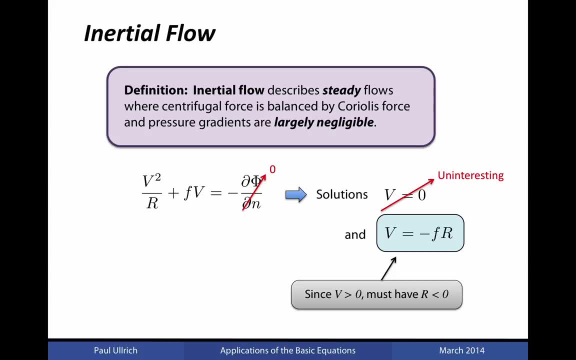 In this case, only the centrifugal force term and the Coriolis force term are retained, and this gives rise to a simple quadratic which has two solutions associated with it, One of which is zero flow speed. so capital V equals zero, which we're going to neglect. 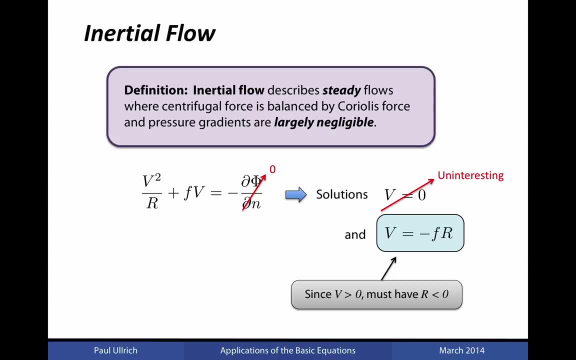 in this case for being uninteresting, And a second solution, which is that the flow speed is equal to negative F times the radius of curvature. Now, since the flow speed must always be positive by construction, we must have that in the northern hemisphere that the radius of curvature must be negative in this case, in order to 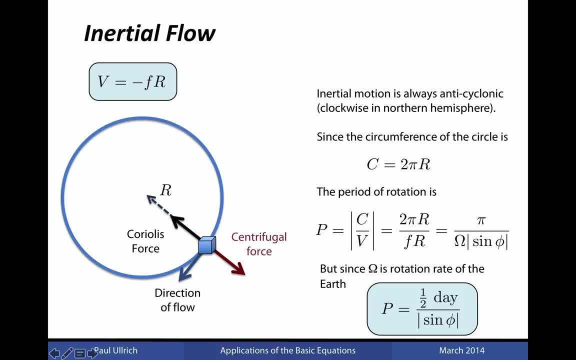 have a physical solution. So for inertial flow with velocity equal to negative F times the radius of curvature, we end up with a force balance diagram analogous to the one depicted here, with centrifugal force directed outward, away from the circle, and Coriolis force directed into the circle. 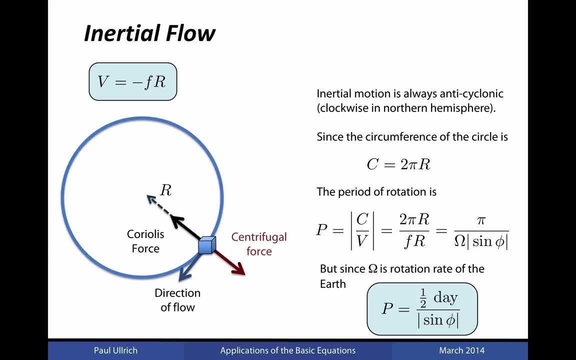 The direction of flow is then clockwise around the circle. The normal vector here is then aligned with the centrifugal force vector. It's always anticyclonic, that is, it's always clockwise in the northern hemisphere and counterclockwise in the southern hemisphere. 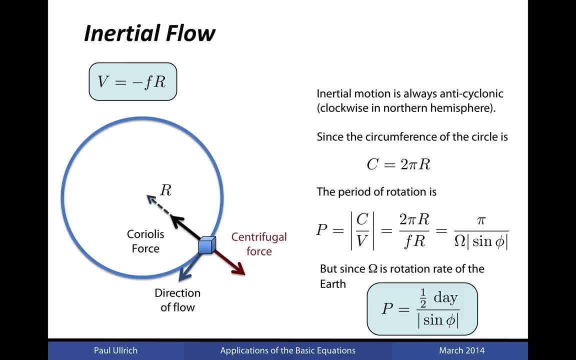 However, we can also, since the flow is circular, we can also derive an expression for the period of rotation associated with the fluid parcel, that is, how long it takes for it to complete one cycle around the circle, Since the circumference of the circle is given by two pi times the radius of curvature and 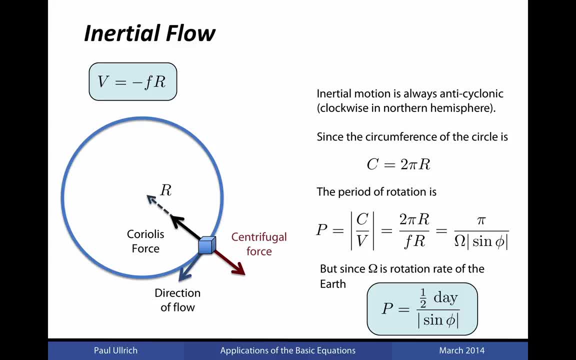 the period of rotation is just going to be equal to length divided by velocity. Then by substituting in the expression for circumference of the circle and the velocity of the fluid parcel, we end up with a period that's equal to pi over omega times, the 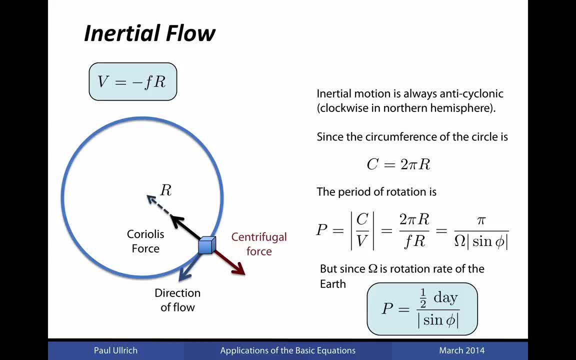 absolute value of the sine of the latitude. Here omega is the rotation rate of the earth, and so is a fixed constant. Consequently, the period is purely a function of the latitude at which the inertial balance occurs. Here omega is the amount of rotation added to the amplitude factor, and so it isそうだ. Уcomm wounded right at the center, just like at the bottom of the circle. So solving ambassadors now isn't just a question of dispersion, but being able to carefully fit棒s appr против the current or protein behavior in order to Спасибо to that. 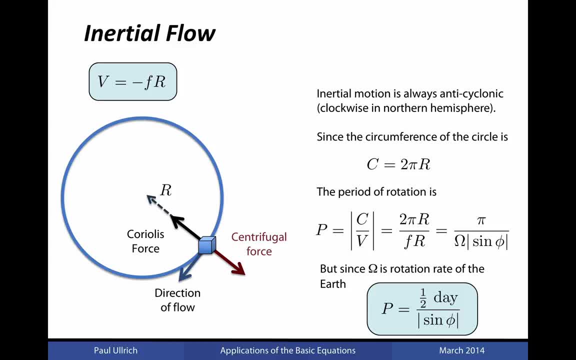 oheah, that's my lab. one half of a day for the value of omega typical for the Earth divided by the absolute value of the sine of the latitude. So you'll notice that because the flow velocity is determined by the strength of the Coriolis force, that as Coriolis force goes to zero, that as we approach the 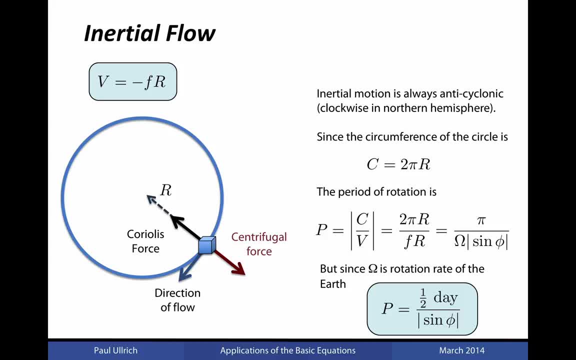 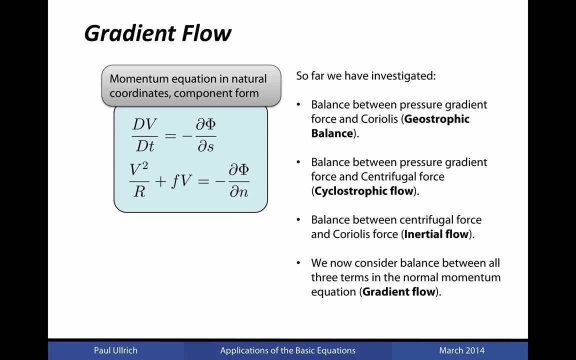 equator, the period of the motion becomes increasingly large, So the period of the rotation becomes large towards the equator and becomes small towards the poles. Let us now consider the general case of gradient flow, which incorporates all three terms in the force-balance. 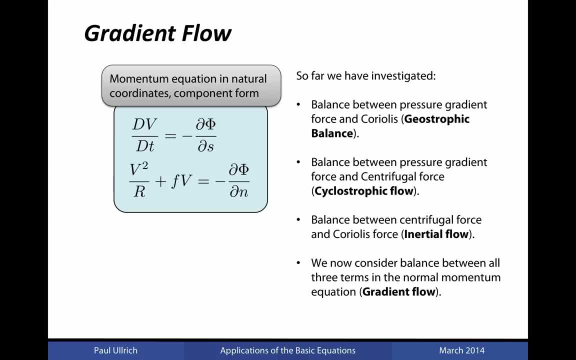 relationship derived using natural coordinates. So far we've considered geostrophic balance, which is Coriolis, and pressure gradient, cyclostrophic flow, which is pressure gradient, and centrifugal and inertial flow, which incorporates centrifugal and Coriolis. The 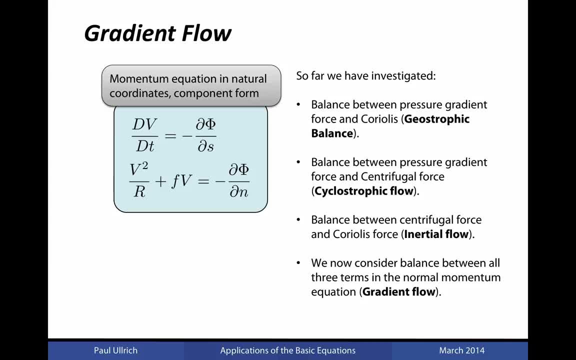 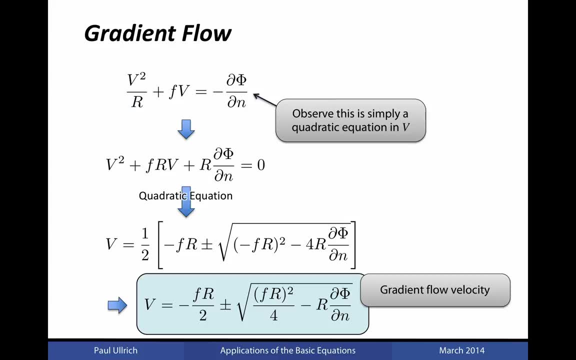 three terms are often pronounced as the same, but they're not the same. So let's look at the present within nature. and so we're interested also in the case where all three terms are relevant towards determining the flow direction. So let's start with our three-term equation. 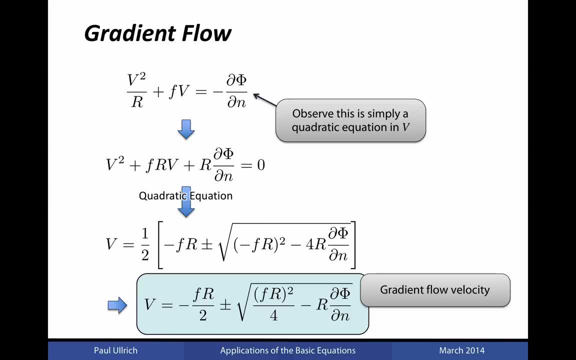 from force-balance, We'll notice that this expression is actually simply a quadratic equation. in the flow velocity v, Again, we are fixing the pressure gradient field, or the geopotential field in this case. so it is prescribed in this equation and kept constant. 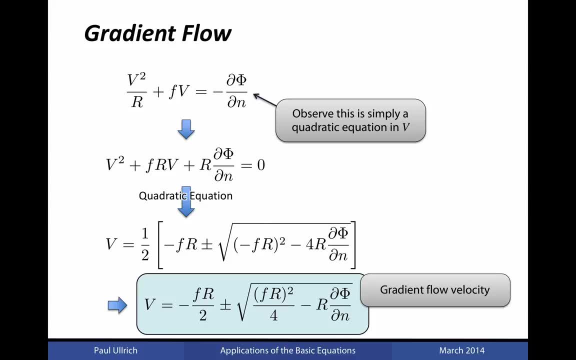 So we're going to look at the flow velocity equation in this case and we're going to look at the flow velocity equation in this case, and we're going to look at the flow velocity equation in this case. We can solve this quadratic equation using typical quadratic formula and arise at a velocity v. 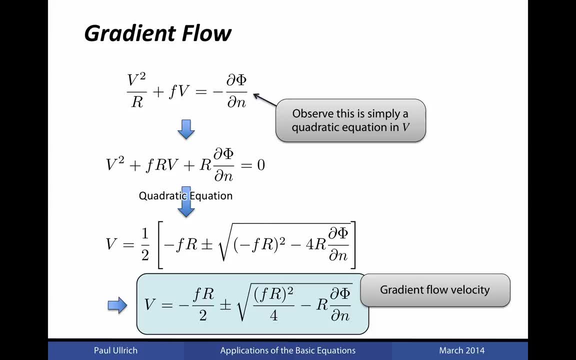 which is given by the expression here. Simplifying this expression gives the expression for the gradient flow velocity shown at the bottom of this slide. Note that not all solutions are possible in this equation. Let's consider the possible choices which arise from different signs associated. 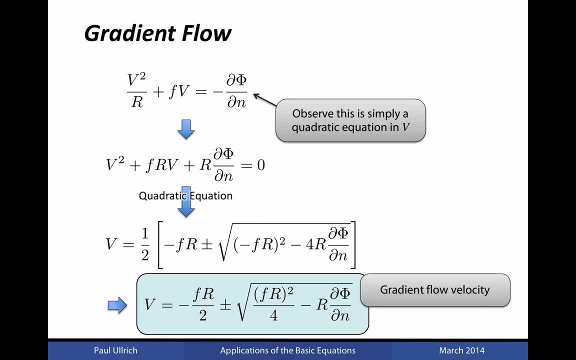 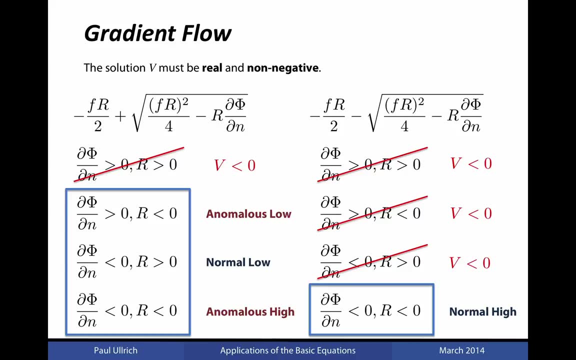 with the pressure, gradient force and the radius of curvature, We know that the solution v must be real and must be non-negative. By construction, we require that this velocity always be non-negative. Consequently, although there are eight cases that arise from different choices of sign in the 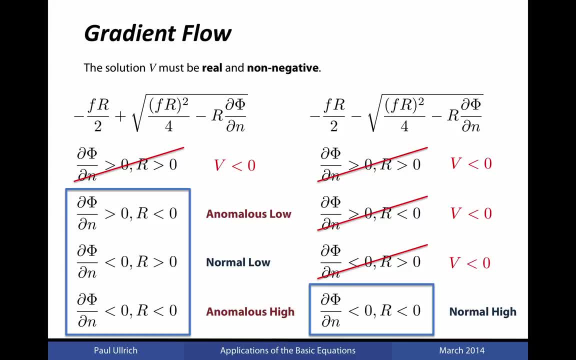 quadratic expression from the previous slide. four of these can actually be eliminated because they give rise to the velocity of the velocity. So we know that the velocity of the velocity is non-negative. Now we can look at the values of the velocity magnitude which are negative. Four of these are actually: 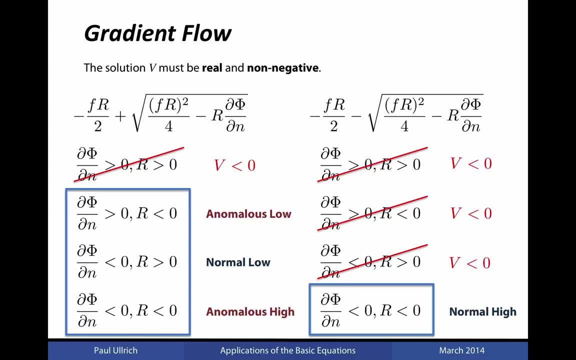 physical solutions and we'll refer to these as normal low, normal high, anomalous low and anomalous high. In the normal low case, it's associated with a derivative of the geopotential field in the normal direction, which is negative, and a positive radius of curvature. For the normal high case, it is: 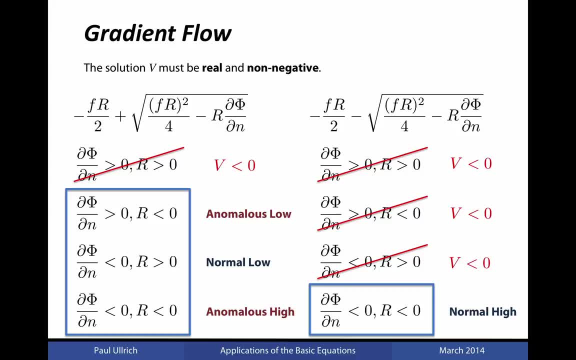 associated with a negative derivative of the geopotential height in the normal direction and negative of the geopotential height in the normal direction. So we know that the velocity of the radius of curvature For the anomalous low case we have a positive. 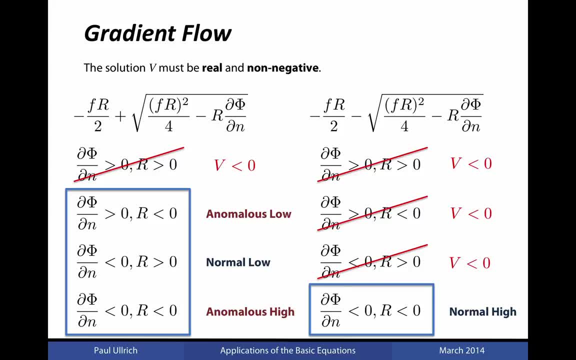 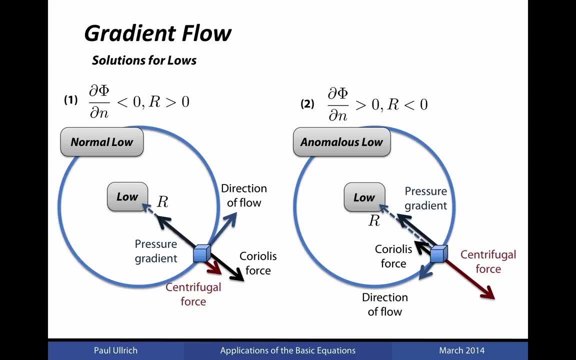 derivative of the geopotential height field in the normal direction and a negative radius of curvature. In the anomalous high case both signs are also negative. So the solution for low pressure fields then look as follows: On the left hand side here we have a normal low and on the right hand side we have 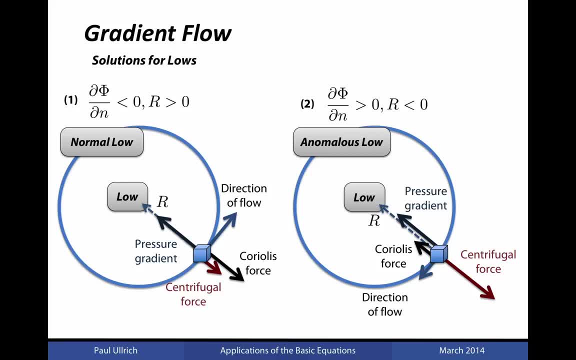 an anomalous low. The normal low is associated with a Coriolis force which is directed outward, away from the direction of curvature, and a centrifugal force which is directed away from the direction of curvature. The pressure gradient force is directed inward, towards the low. The sum of the Coriolis 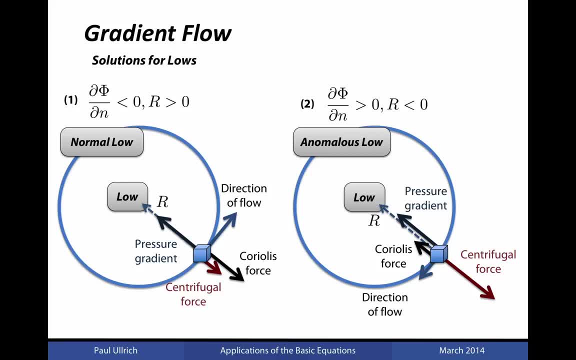 force and centrifugal force in this case must balance that pressure gradient force and consequently we observe a counterclockwise rotation of the flow around the central low. In the case of an anomalous low, we have that the centrifugal force is significantly stronger than the Coriolis force. This allows the Coriolis force to 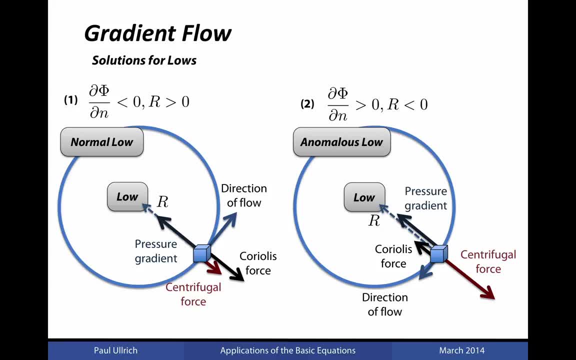 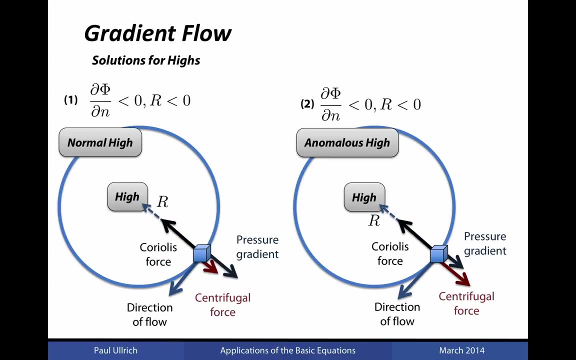 be directed inward and allows for the fluid parcel to be moving in an anticyclonic direction. In this case, the pressure gradient is again directed inward towards the low, along with Coriolis force, and these two are balanced by the centrifugal force directed outward. The solution for highs are given. 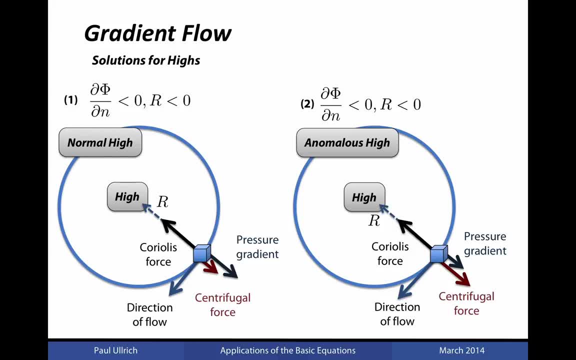 here The left hand side shows the normal high and the right hand side shows the anomalous high. These two highs are actually identical to one another, except for the magnitude of the centrifugal force relative to the pressure gradient force. For a normal high, the centrifugal force is much weaker than the pressure gradient force. 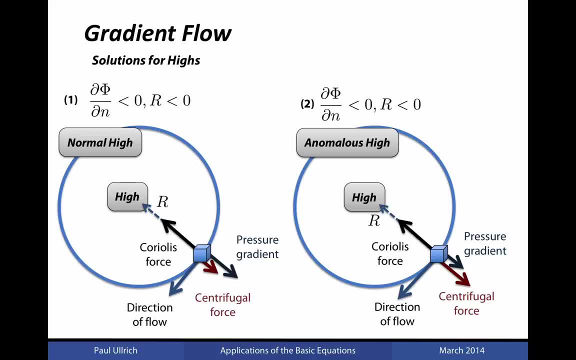 This is assumed. this arises naturally from the case where you have weak curvature associated with the flow. The anomalous high case occurs when you have strong curvature associated with the flow, such that the centrifugal force is actually greater in magnitude than the pressure gradient force. 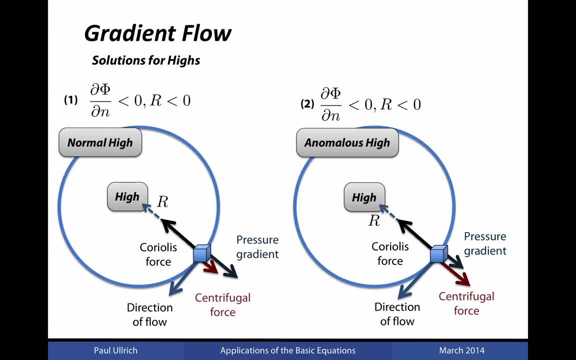 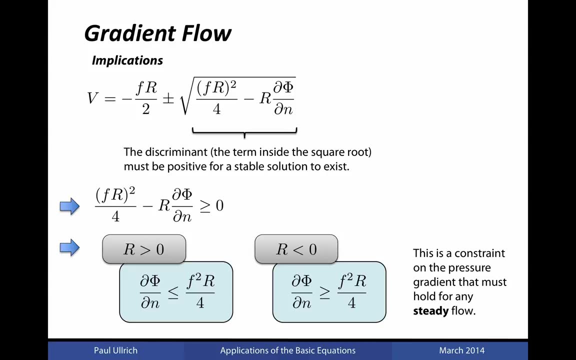 In both cases, we have a pressure gradient which is directed outward, away from the high, and this is balanced by a Coriolis force which is directed inward. Unlike the case for low pressure systems, the direction of flow is always clockwise. So what are the implications of this solution then? We know that the 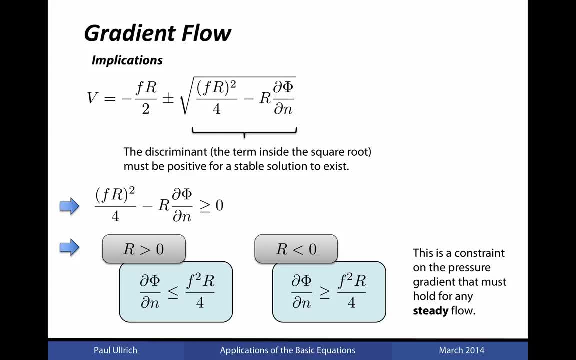 discriminant, which is the term that appears within the square root of the velocity solution for gradient flow must be positive in order for stable solutions to exist. That is, we must have a real value of the square root and not an imaginary value for the solution to. 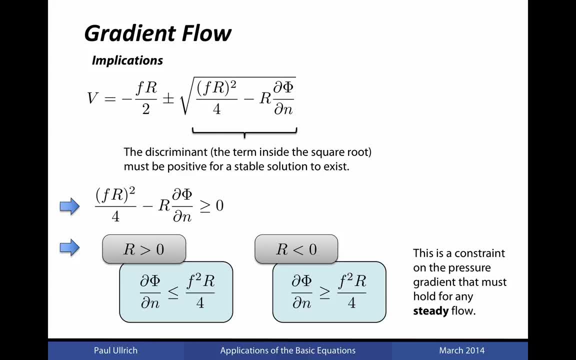 be physical. This then implies that the interior term must be greater than or equal to zero, or not negative. There are, then, two cases that you can observe that arise from this inequality. One is for the case of positive radius of curvature, in which case the derivative of the geopotential height 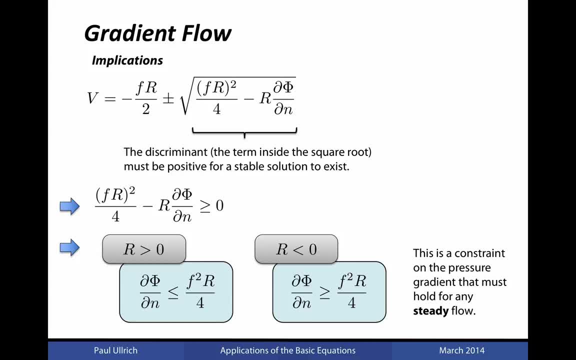 field in the normal direction must be less than or equal to F squared R over 4. and in the case of a negative radius of curvature, we then have that the derivative of the geopotential height field in the normal direction must be greater than or equal to F squared R over 4.. So this is a constraint that must. 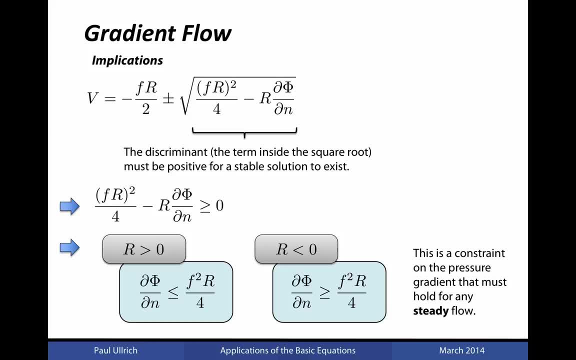 hold for any steady flow and it's a constraint that must hold on the pressure gradient field. If this constraint does not hold, then the flow cannot be in a steady balance. The flow is not a constant state and will instead fall apart and produce a more chaotic solution or time dependent solution. 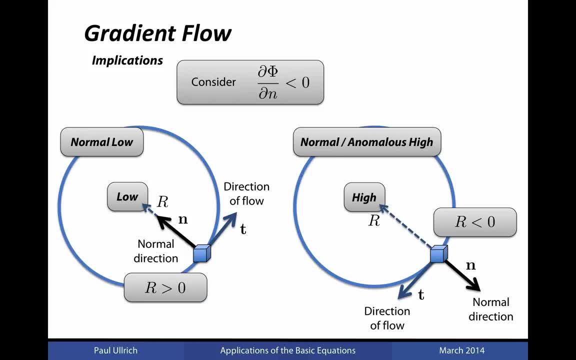 OK, for the case of a normal low. let's consider how this inequality plays out On the left-hand side. we have a radius of curvature which is positive. direction of flow is counterclockwise around the low. normal direction is pointed into the low-pressure region and aligned with the radius of curvature. This is a typical. 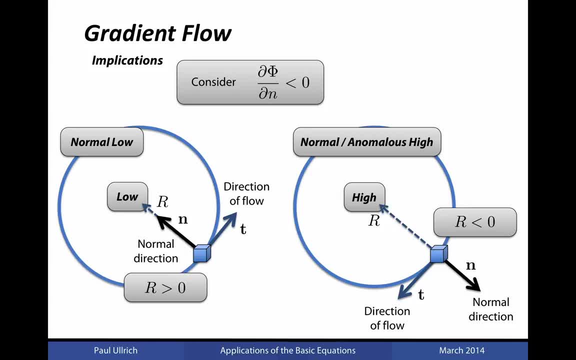 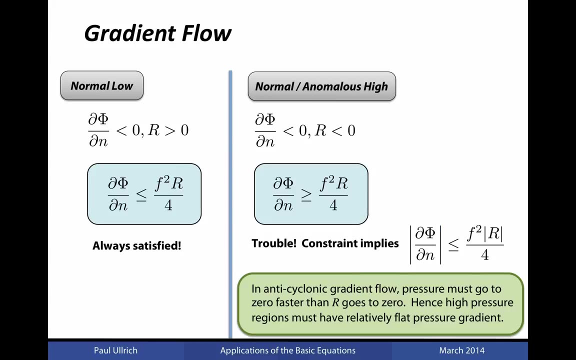 normal low configuration. On the right-hand side, we have our normal and anomalous high, both of which share an identical configuration where the flow is in the clockwise direction about the high, with a normal directed outward and hence a negative radius of curvature. For the normal low case we have that the 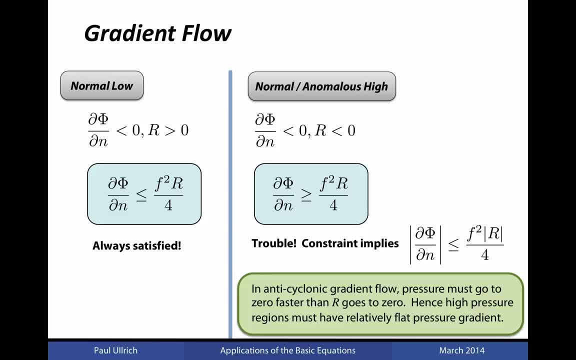 derivative of the geopotential height field in the normal direction is negative and the radius of curvature is positive. Consequently, we then have that the right-hand side of this inequality is always positive, whereas the left-hand side is always negative, and so the inequality is always. 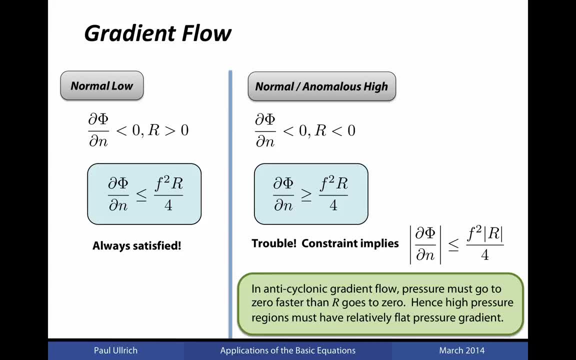 satisfied, regardless of the strength of the pressure gradient. In the case of a normal or anomalous high, both terms are negative, and so we actually have a constraint that then arises on the pressure gradient field in terms of the radius of curvature, in order to maintain a steady flow. In fact, this 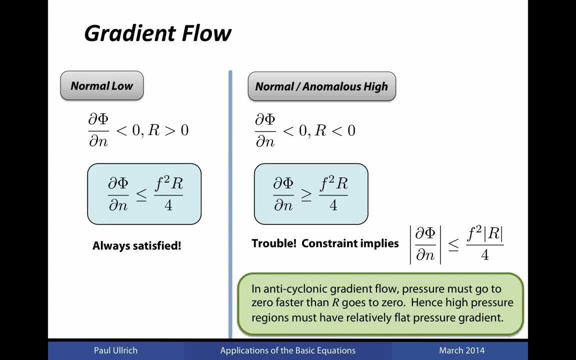 constraint implies, the absolute value of the derivative of the geopotential height field in the normal direction must be less than or equal to F squared times the absolute value of the radius of curvature divided by 4.. If you consider now a series of concentric circles corresponding to fluid parcels, 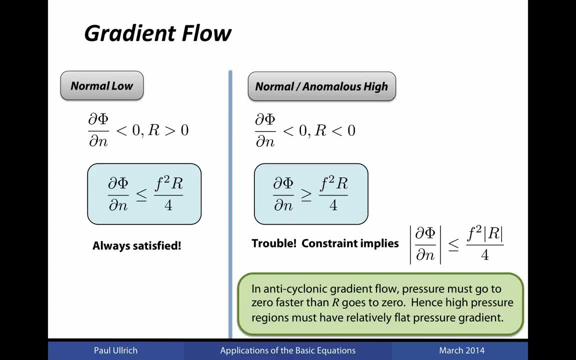 which are rotating about the high. as you get closer and closer to the center of the high, you will have a radius of curvature which goes to zero as you are approaching the center of the circle. This constraint then implies that the pressure gradient must go to zero faster than the radius of curvature goes to. 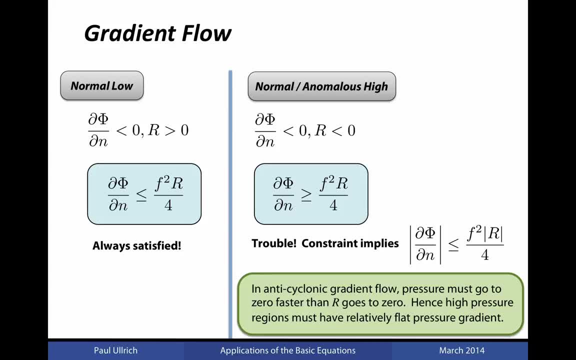 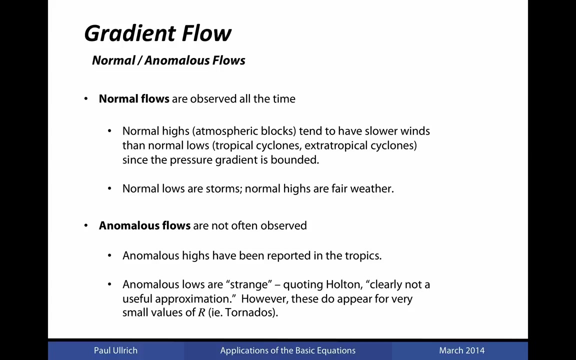 zero and so provides an intrinsic constraint on the maximum strength of the pressure gradient as you approach the interior of the high. Consequently, high pressure regions must have relatively flat pressure gradients on their interior, which is not required for the case of low pressure regions. As a result, we actually have that normal highs tend to have slower wind speeds. 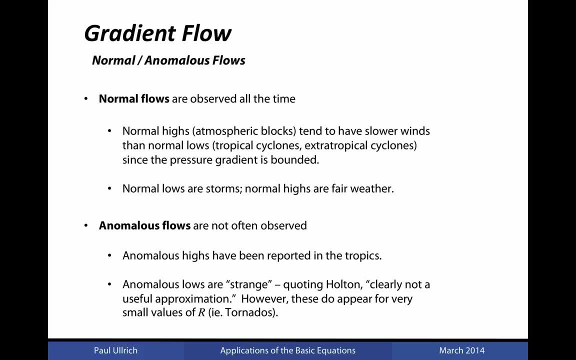 than normal lows because the pressure gradient force is bounded and are typically then associated with fair weather. Normal lows which do not have any such constraint can have very strong pressure gradients towards the interior and consequently can give rise to strong storm systems. Hence we claim normal lows. 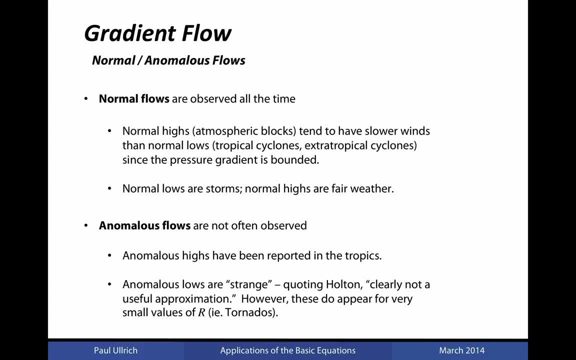 are storms and hence normal highs are fair weather. Anomalous flows were not touched on in too much detail in this lecture, but they're not often observed in nature. For most large-scale motion, normal lows and normal highs are the dominant flow pattern. With that said, anomalous highs. 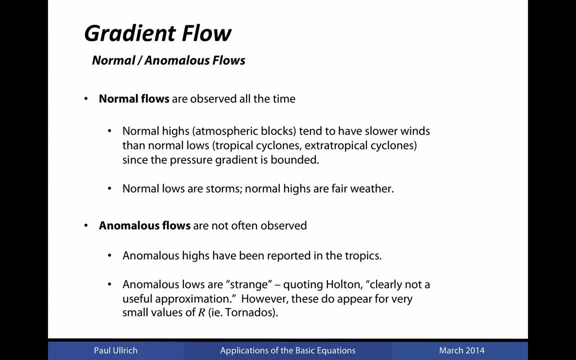 have been reported in the tropics, and they are a physical solution of the gradient flow equations. But anomalous lows, on the other hand, are considered strange and often not a useful approximation. However, with that said, they do appear in the case for very, very small values of the radius of